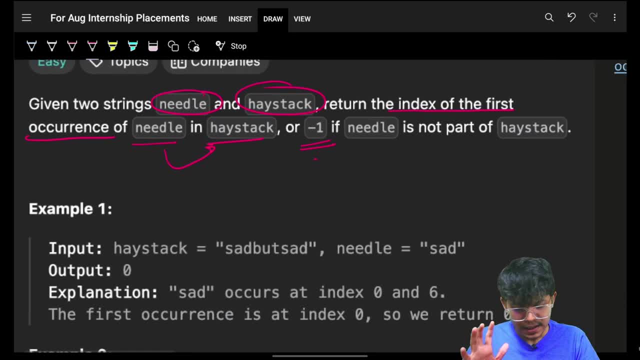 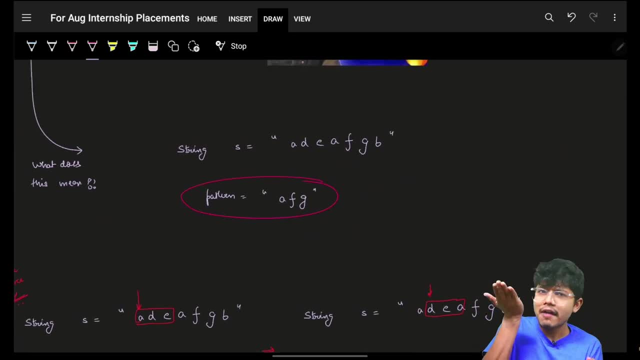 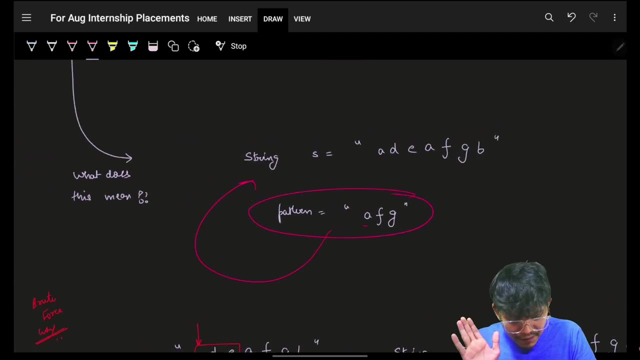 And if it's possible brute force, then for sure. brute force is always there for us. But we will see that if we go about in a brute force manner. consider again: it's just that we have a pattern and we have to search that pattern in a string. So, taking the simple example of searching a pattern in our string, So we have AFG. I have to search this AFG. I can easily see the first occurrence of AFG in my string. S is at this location. So I have to return the index 0, 1, 2 and 3.. I return the index 3.. 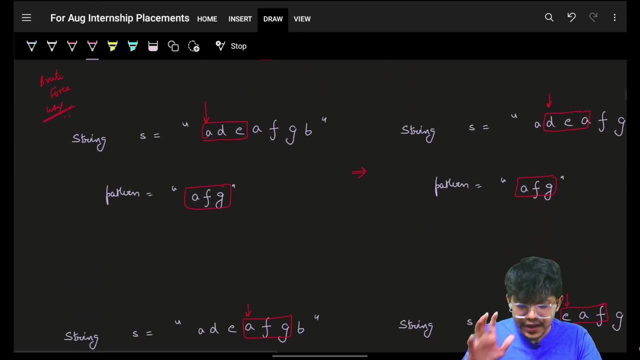 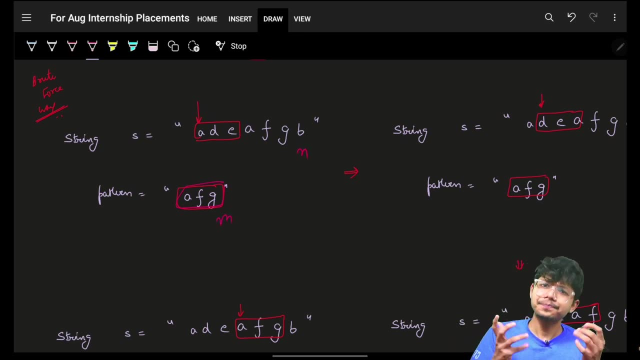 If I'm not able to find it, I simply return the minus 1.. So very brute force technique says that you have this string of size M, You have the upper string of size N, which is the string S main string. You will compare the entire string of length M, starting from this index. Compare the entire string. 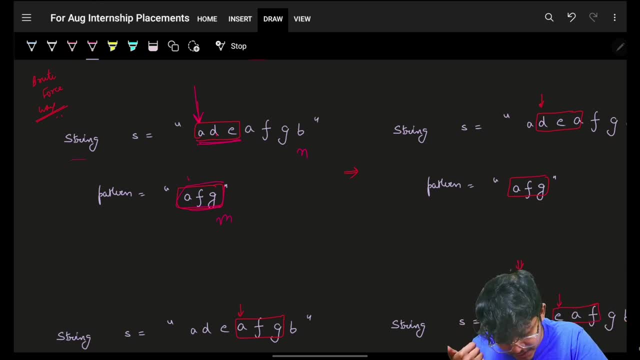 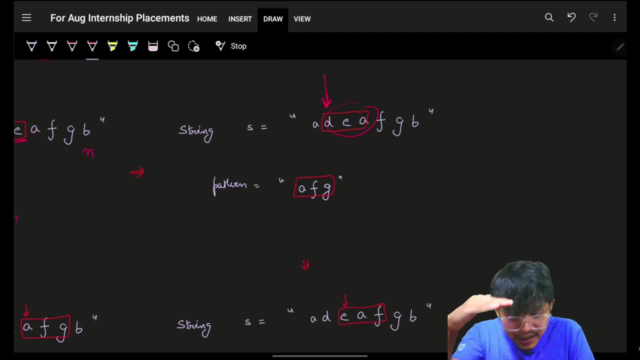 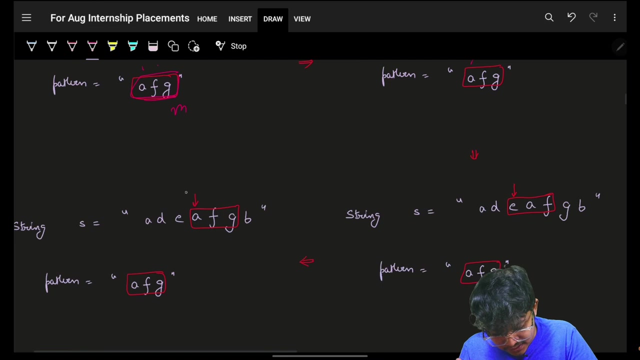 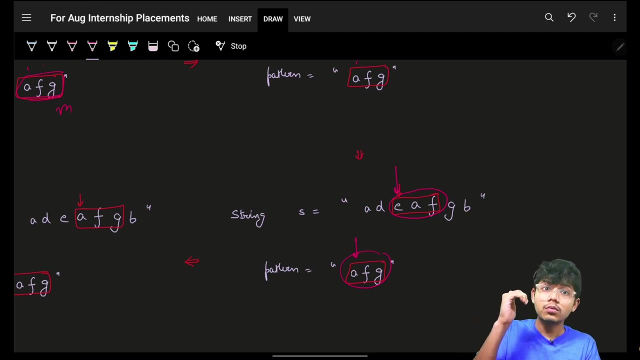 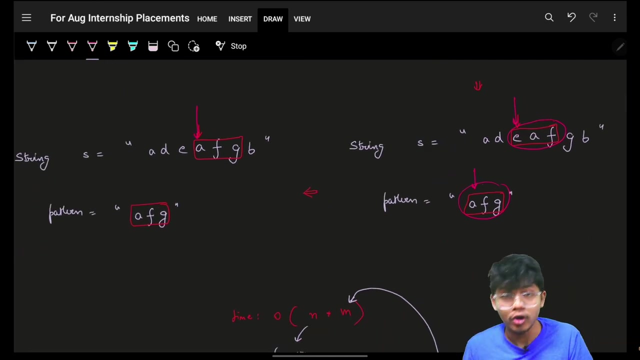 I'll compare A, Okay, matched. Compare D: Ah, not matched. Cool, No worries, Now go on. Now I will go on and compare the entire string of length M again, And the entire pattern: Okay, A, A matched. No, it's not matching. Okay, No worries, Now, next, Okay, Next, I'll move on. I'll compare the entire string E, A, F, G with A, F, G. You will see, Oh, compare, compare, compare. Oh, oh, At E and A it was not matching. So I simply moved on. Okay, I moved on here. Then I was here Again. compare the pattern: A, A matched. Okay, F, F matched. Okay, G, G matched. Oh, entire pattern is matching. So you will say: okay, Aryan. that's, I can simply say. 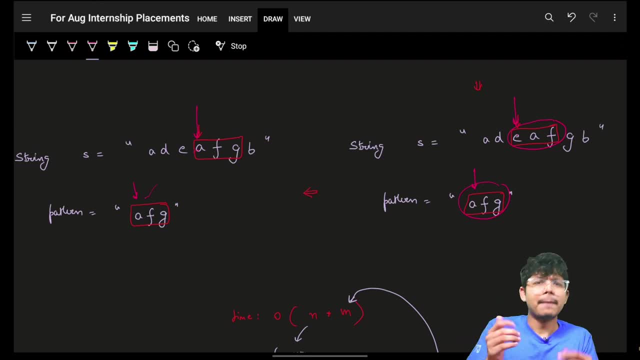 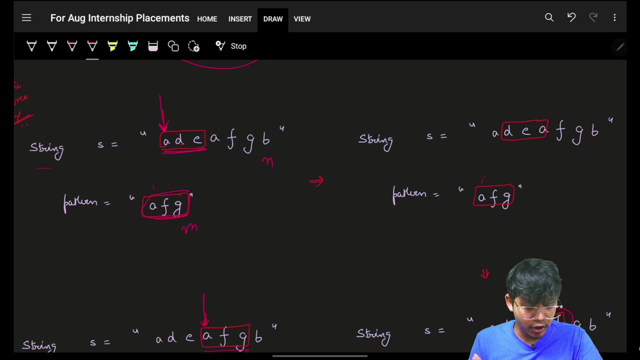 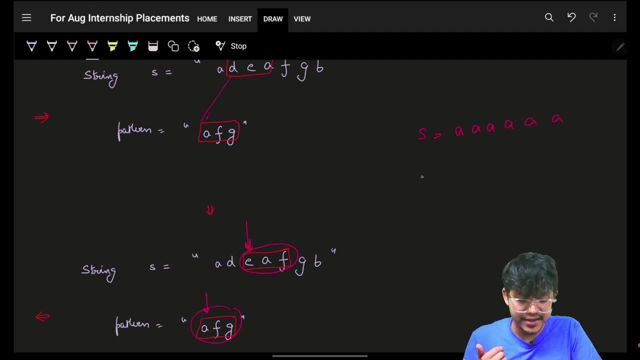 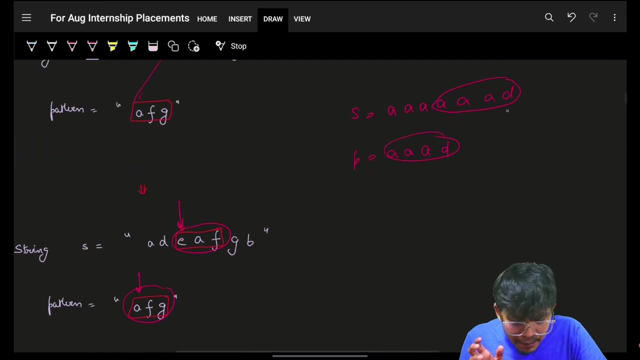 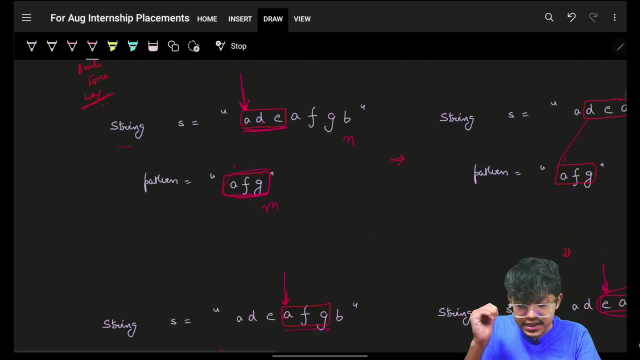 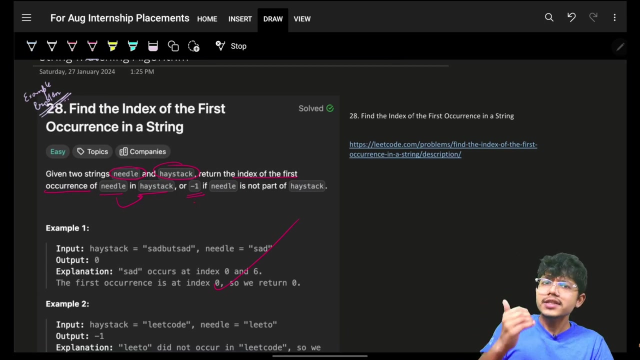 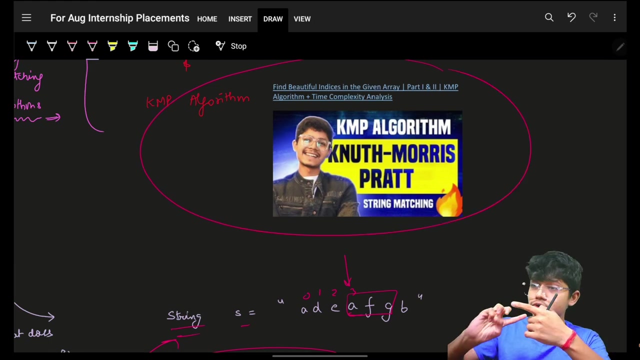 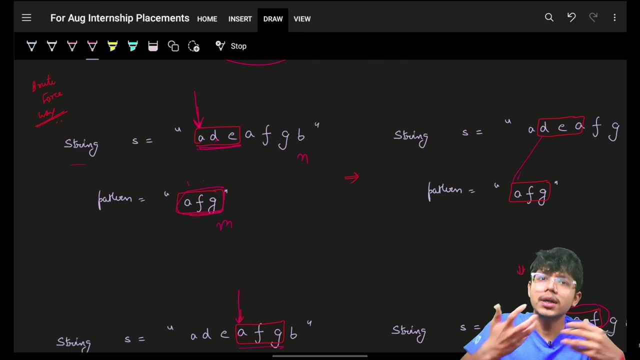 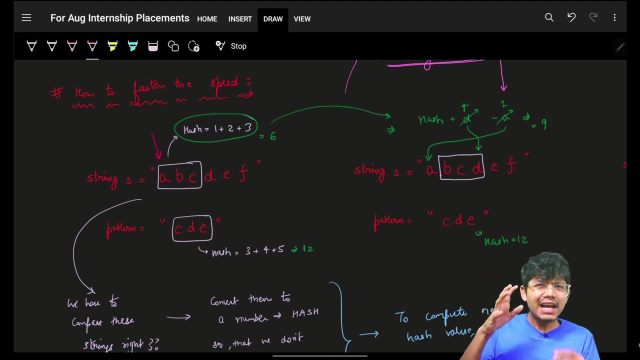 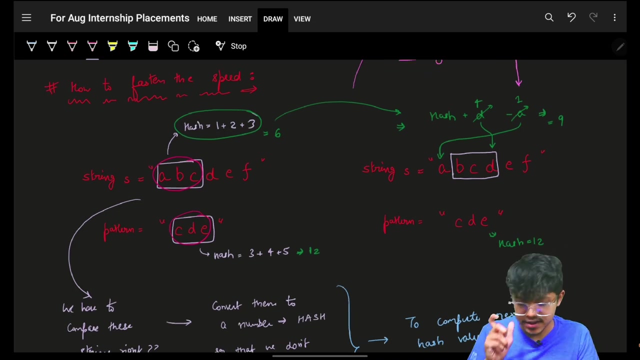 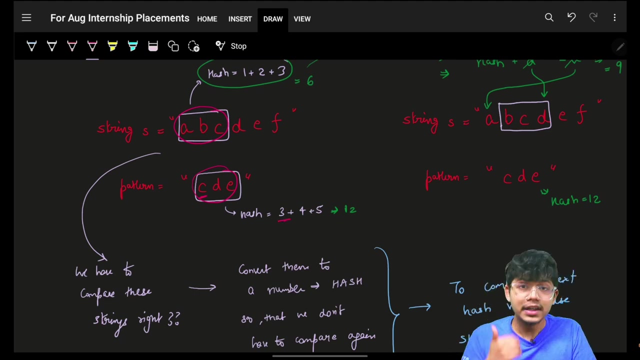 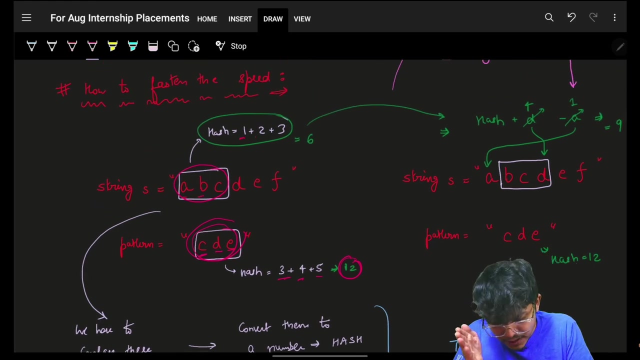 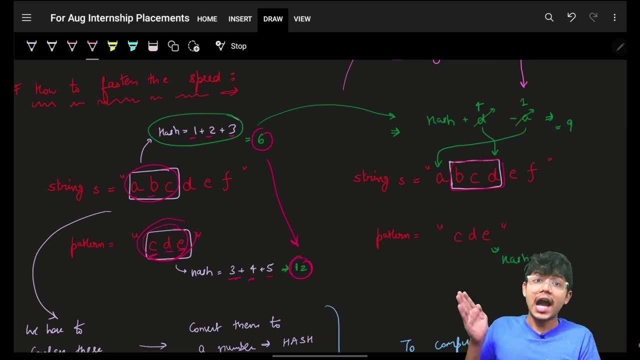 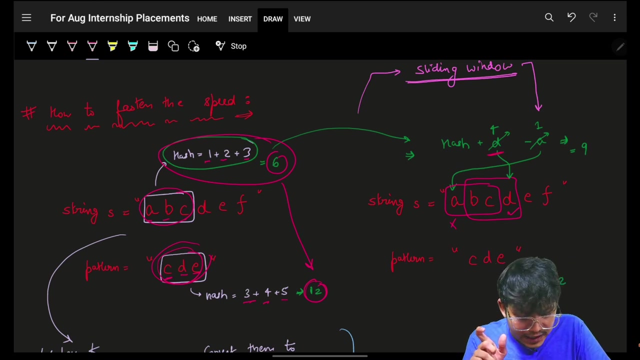 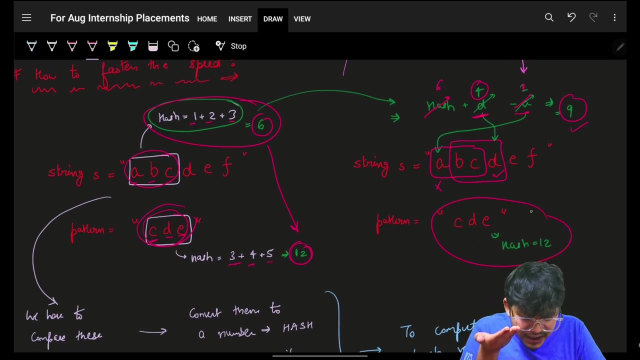 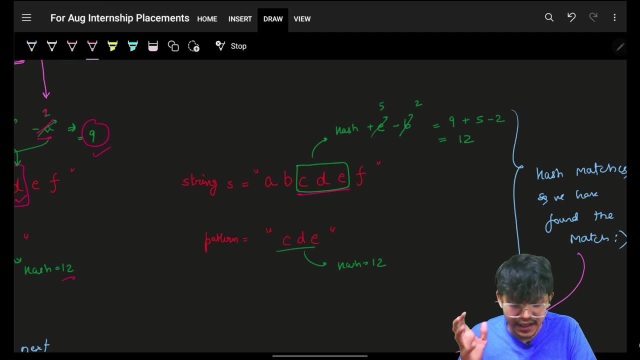 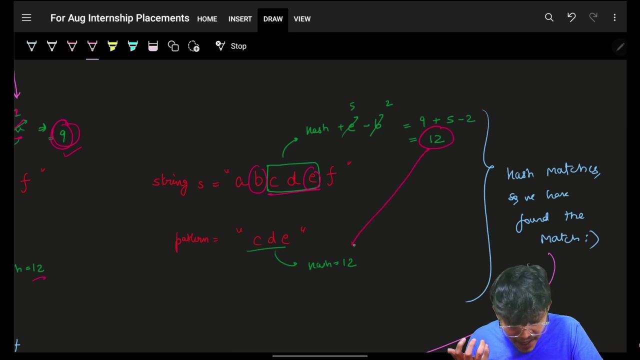 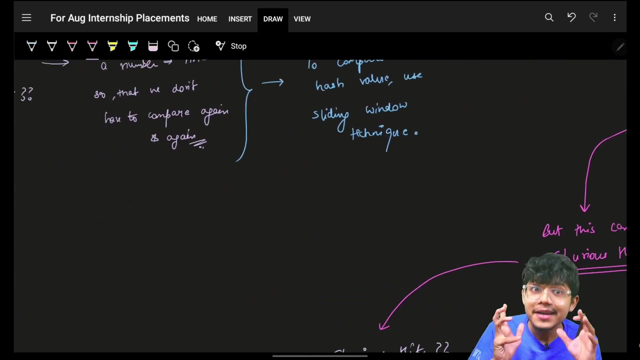 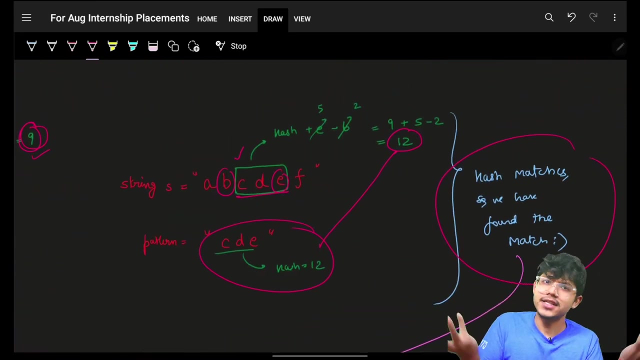 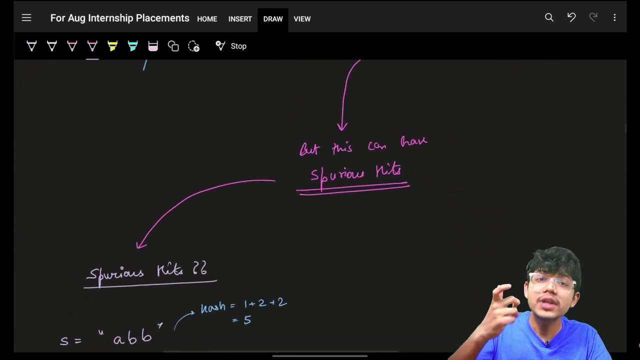 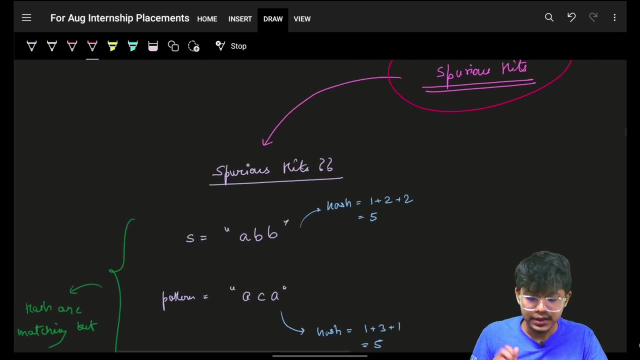 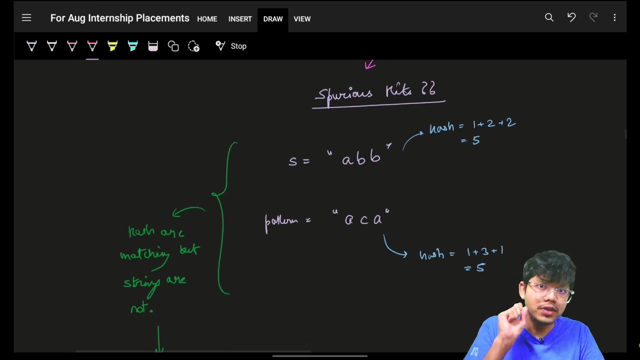 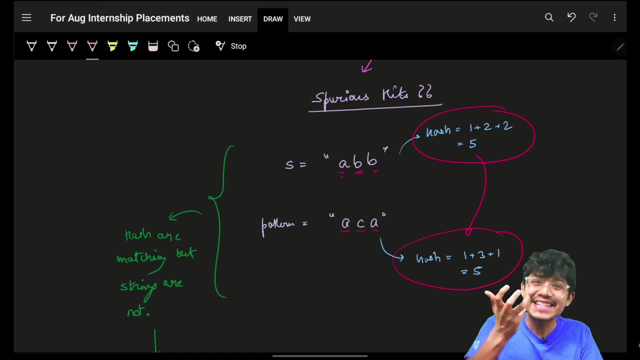 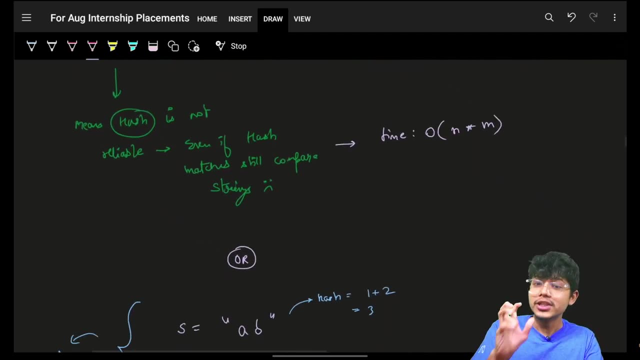 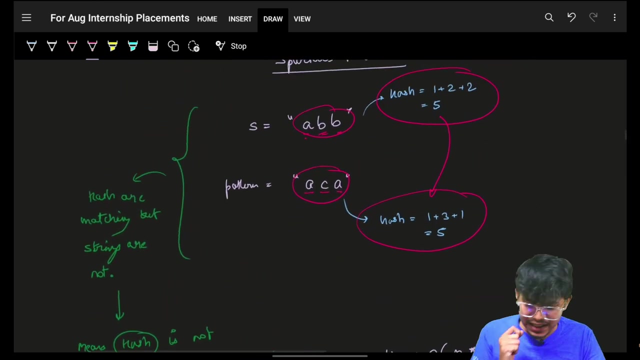 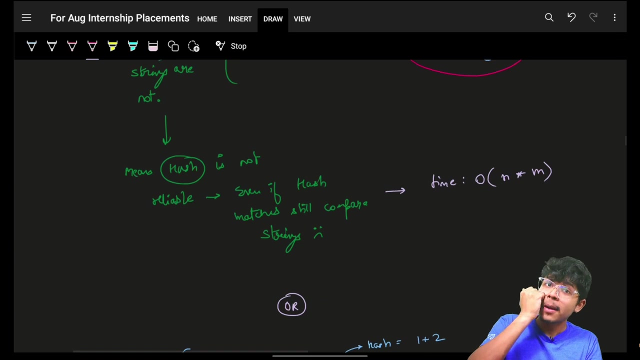 you will infer, strings are also same. But, bro, you can easily see A, B, B is not equal to A, C, A, Which means your hashes are not good. So now I saw: oh, even if, even if I match a hash, then still I have to go and compare the actual strings to know if they are matching or not. So again the time complexity which I was thinking might have gone to O of N plus M, Still it has come to O of N into M because of those spurious hits. 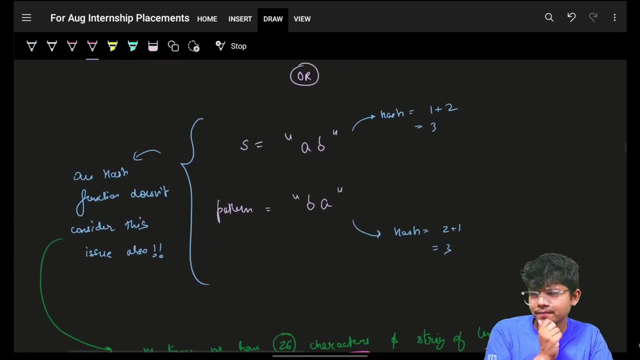 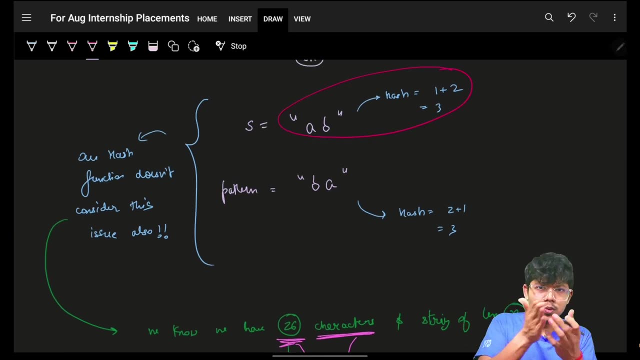 Spurious hits. What can I do for this? That's a thing for us to think of, that, what we can do Again. another example we can see: The hash for this is 3, A- B, But the hash for B also will be same. 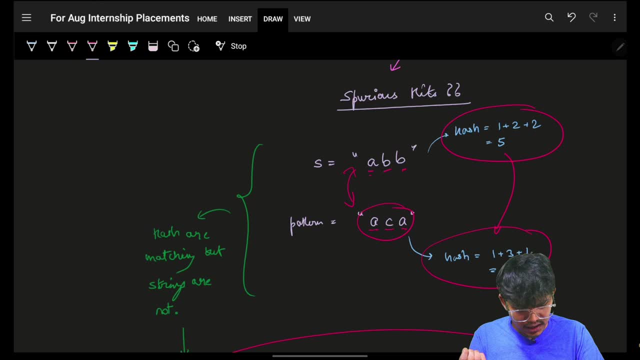 So what we can infer, Like one thing we can infer is: okay, the characters were different, But maybe I can repeat the character. Let's say B, B was repeated, But then a higher character and then a lower character. 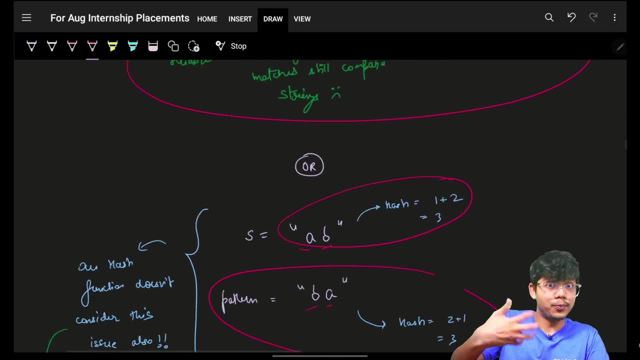 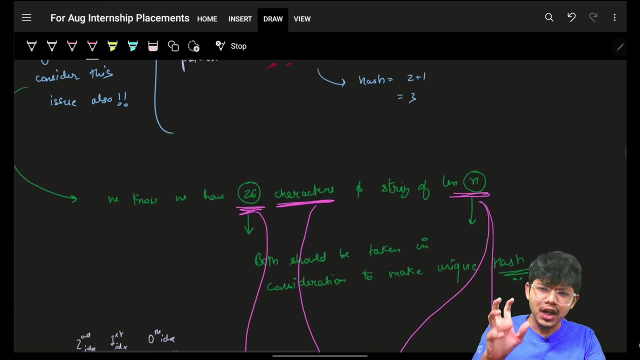 So balancing was there Okay. because of that I was getting spurious hits. What if I had different arrangement? A, B, B, A Order also matters, Oh, so what I figured out was okay. I have 26 characters. 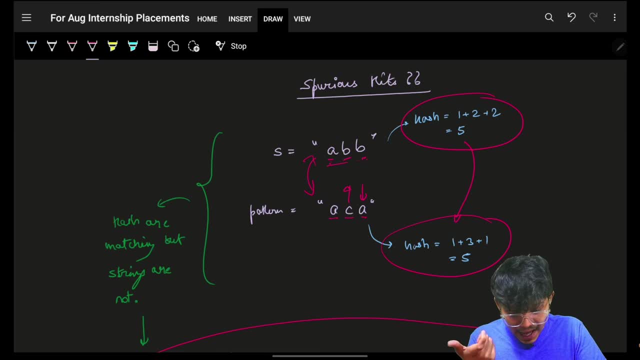 So that's one thing which will matter, because you saw, having a A, B, B, having a A C, A, Which means if I had a C, one more character, B, other character. So for me number of characters will matter. 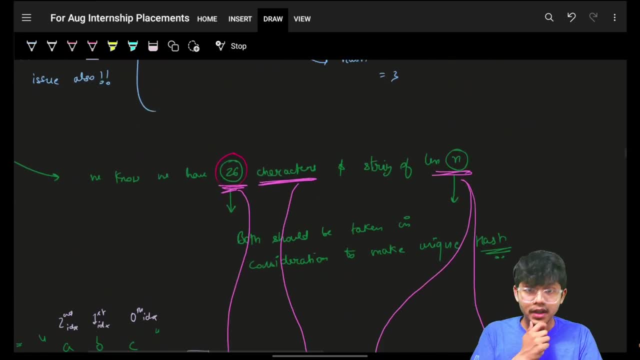 If I have how many characters I have, Okay. Also, it matters what character I have. All right, C versus. okay, I have, let's say, two characters. I have, let's say, two characters: A, B. I have A, C matters. 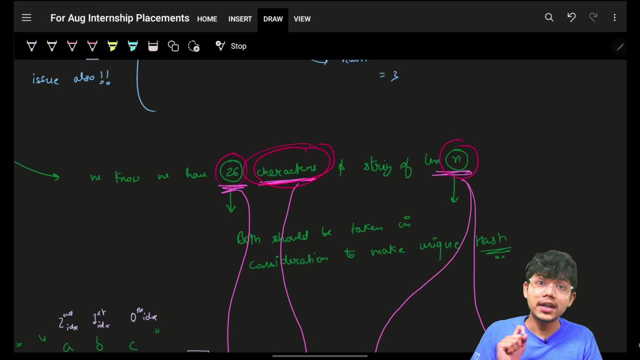 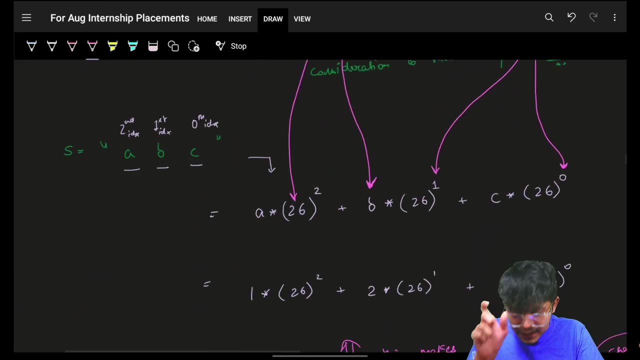 So characters also matters And the length also will matter. How big the length is, I mean you are saying, because you know that part, How would I know it matters or not? See, if I ask you, if you had a string, you have to make a unique hash for it. 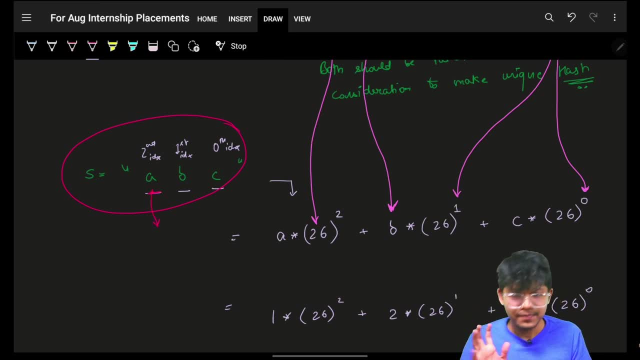 Now, one thing I was doing is I was inferring this A and I was saying: bro A is there? Bro A is there. Then I will say: A's hash is one, B's hash is two, C's hash is three. 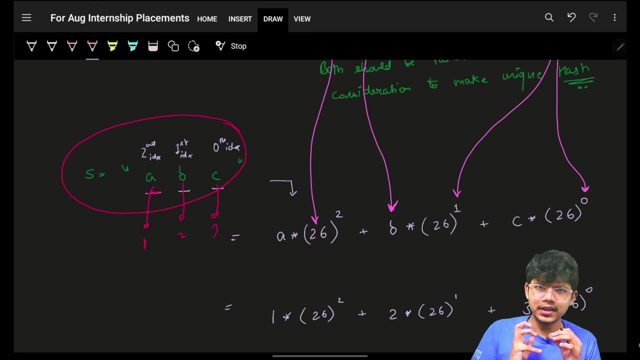 Now let's say I have A, So I was saying this factor. right Now I'll go and ask you What you have to do is you have to uniquely say that at this specific index again, if I put the indexes from the super end, so index zero, index one, index two: 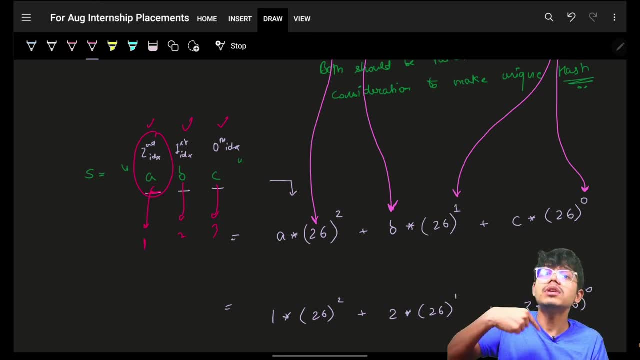 At the index two, I have A. I have to figure out that part. So I'll say: at index two, at index two, I have A. OK, but then what is this? What is this factor? Why is this factor required? 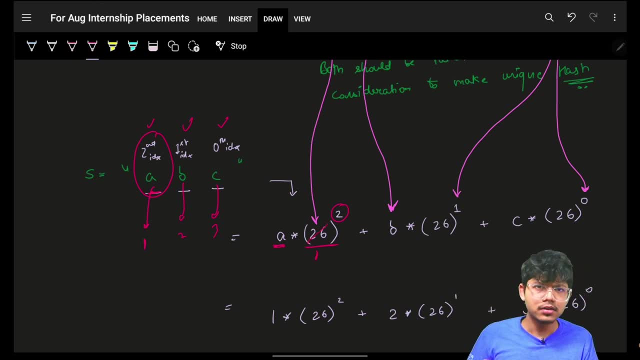 Why can't I put any number? Let's say one. I can't put a one. Why? Why can't I put a one? OK, I mean, one square might give us the same value, So why can't I put a two? 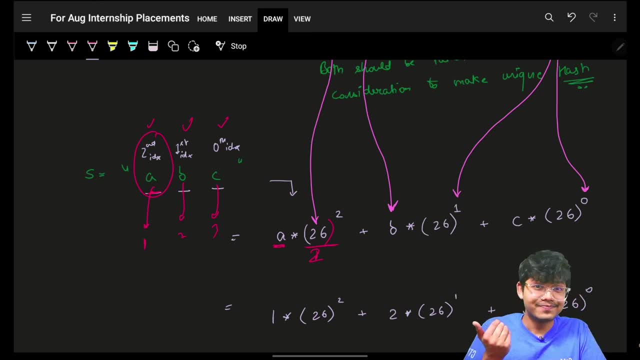 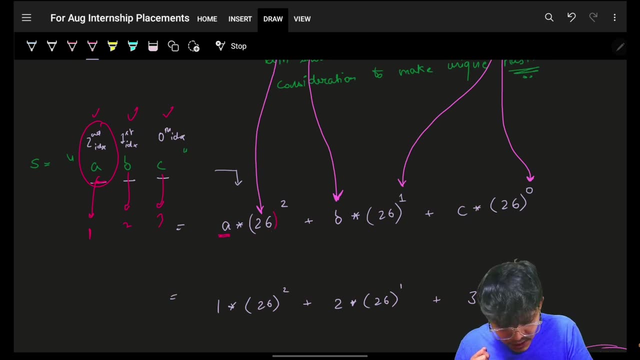 That's also OK, completely fine, right. Because no? no, because if I put a two here? for example, let's say, if you would have put a two here, what would have happened If you would have put a two here? 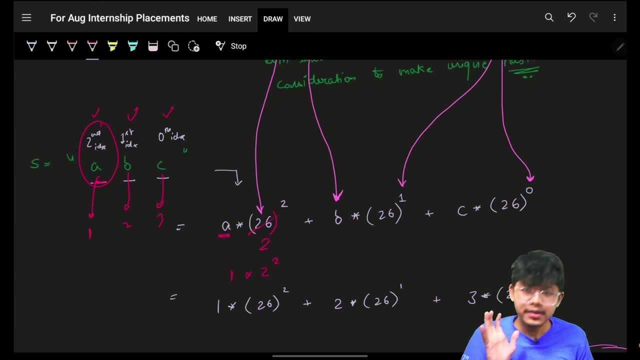 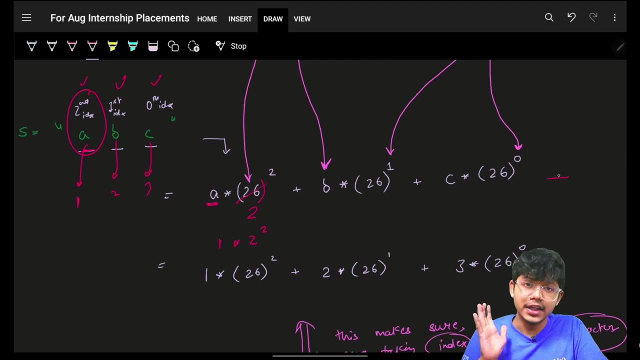 then you would have got a two square multiplied by, let's say, one. OK, A value is one. Then what if I ask you if I would have some previous value? some previous value? let's say, here is a two, two. 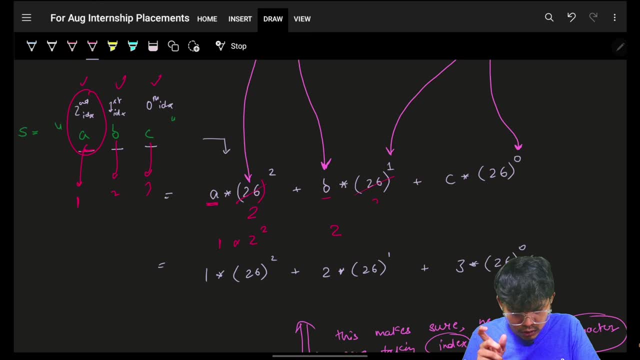 then you would have said hash like this: base factor will be two, So here will be two multiplied by two, So it will also form two square. It will also form two square. You are gone. So why was this required? So I have to put some. 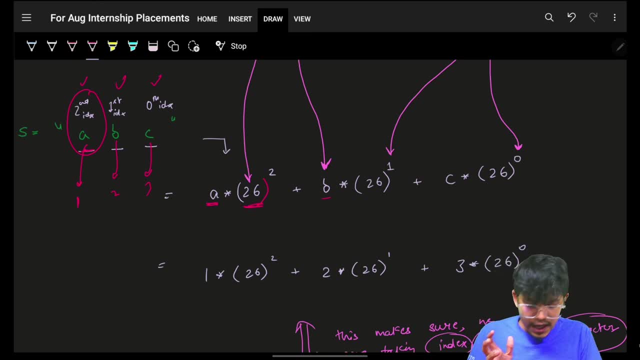 base value, some base value, such that everyone, everyone, no matter what is multiplied to them, no matter what is multiplied to them, they should not become equal to anyone else. That's, that's my prime name, So I have to put in again: 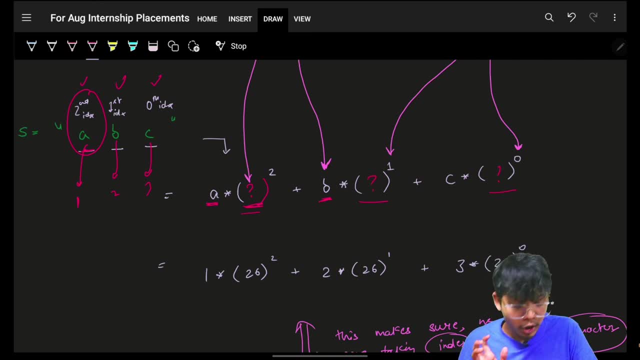 That's a question mark for me. That's a question mark for me. That's a question mark for me: What to put in as a base. I will put in something, no matter what I multiply here Again, what I'm multiplying here, I'm multiplying the characters. 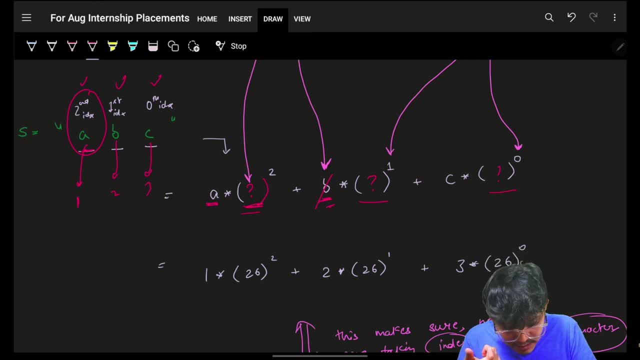 I know the characters from A to Z, which means the maximum number I can multiply. here is a twenty five. Right, I can say A, I can say zero And for Z I can say twenty five. Maybe earlier I was doing a one, two, three. 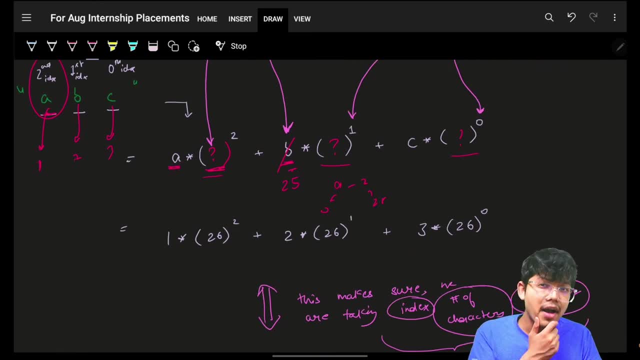 I can say from zero to twenty five also. So I saw, maximum I can multiply is twenty five. So I should put a factor here such that it is more than twenty five. I can put hundred, That's completely fine. I can put a twenty six, twenty seven. 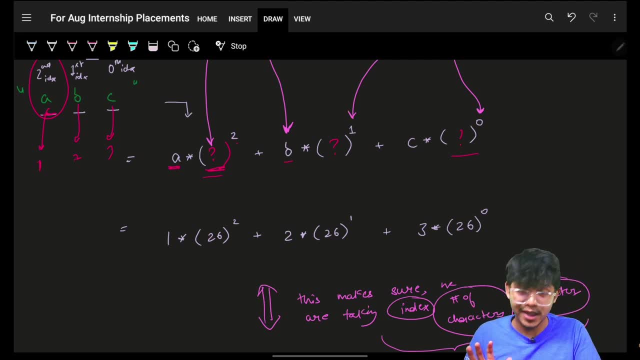 I can put anything I want. OK, I don't know, because the things are being squaring up, So number can become very large. That's also a pain to me, So I'll put minimum value: OK twenty six, OK, twenty six. 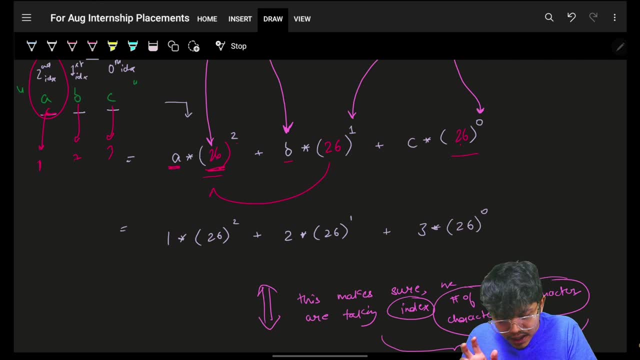 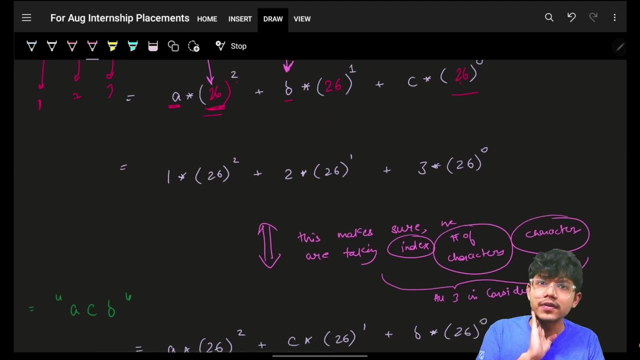 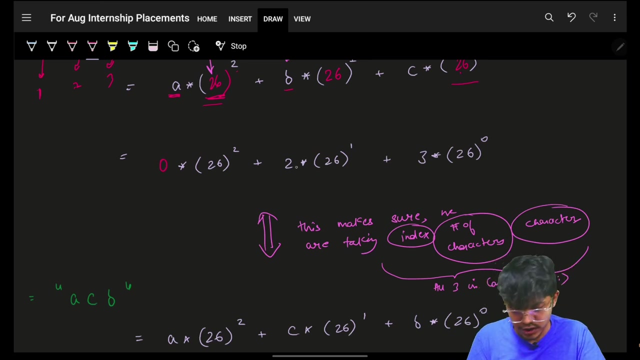 OK, twenty six, So that nothing will actually hamper each other, Nothing will hamper each other out. OK, great, Seems fine, Seems fine. So what will happen is again Usually, like you will see later on, going forward: A, we actually hash to zero, then B to one, and then C and so on and so forth. 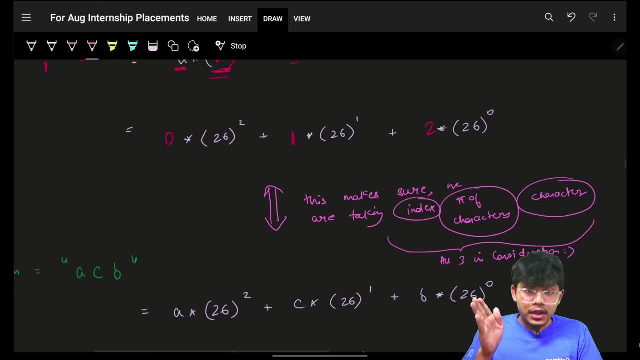 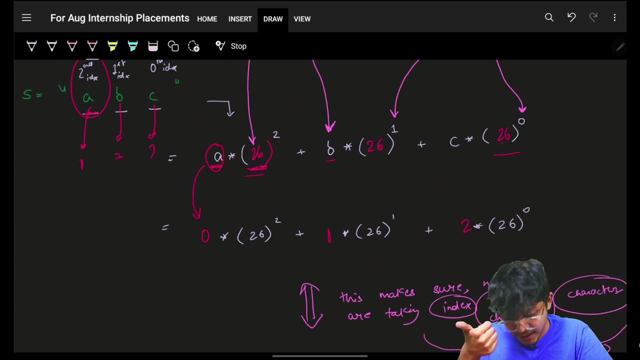 So as to become, like to make it more consistent. Now, OK, that seems completely fine that we had made sure that we are taking the character, which means I'm converting the character and converting and using the location and to not avoid, like to avoid, actually hitting each other. 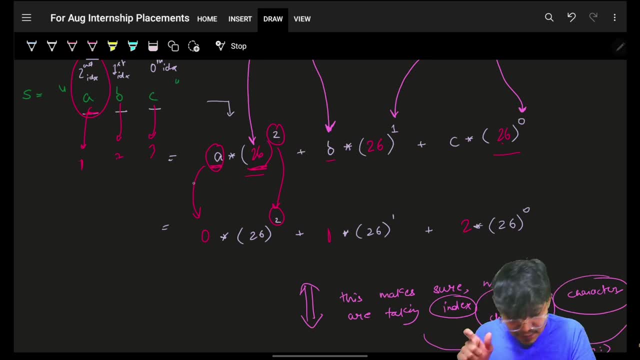 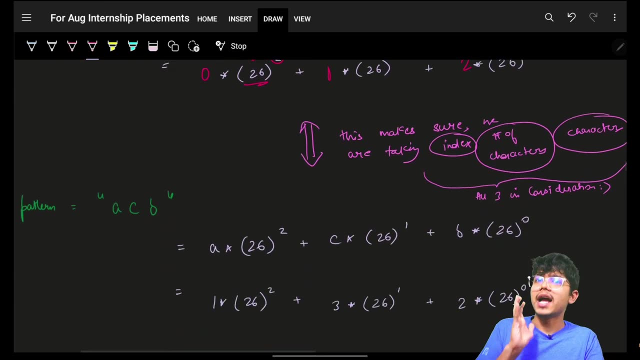 which means these might hit each other so as to make this specific thing. I am having the maximum factor here, which is twenty six. So I need these three things to actually make my hash function to be very unique. So I figure out one thing that I will make my hash function like this: 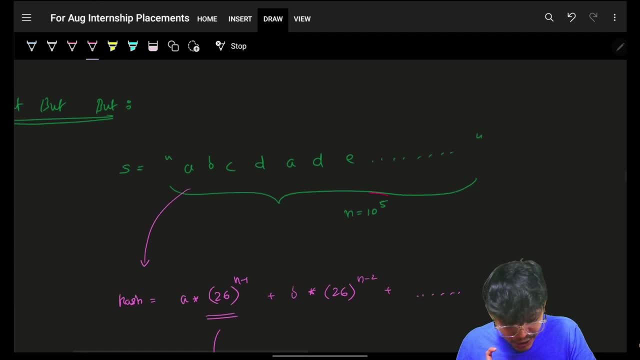 That's going to be super unique, But but, but you saw that you're in. the value usually can go to one in five, which means you have, you can have one in five number of characters, which means this in index value can also go to one in five roughly. 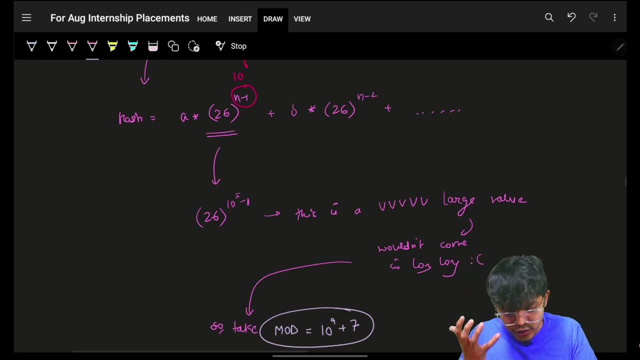 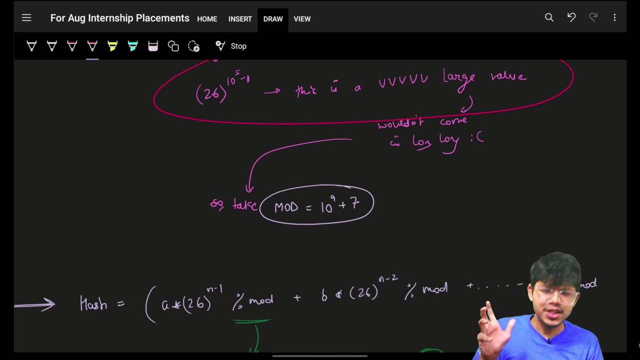 So twenty six, That's going to be a very, very, very large number that you cannot store in your integers, or even long, longs, not even in any possible way. So then you cannot store something very large. You have one operation which is modulo with a prime number. 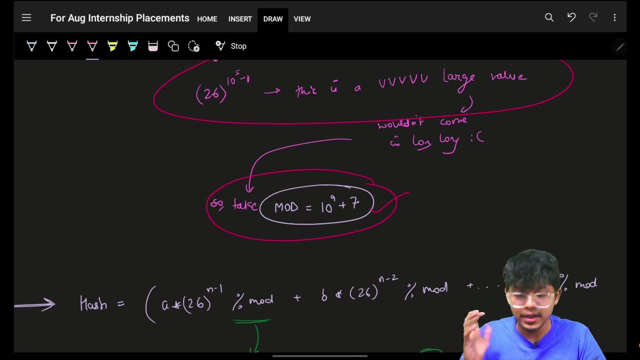 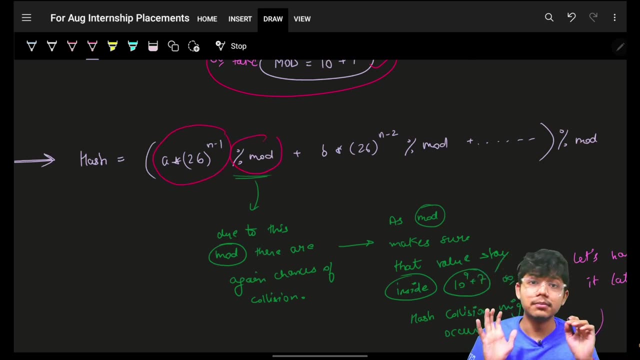 So you usually do one thing to a modulo with a prime number. So that's something. I know that this value can go very large, So I'll do a modulo with a prime number. I know this value can go very large, I'll do a modulo with a prime number. 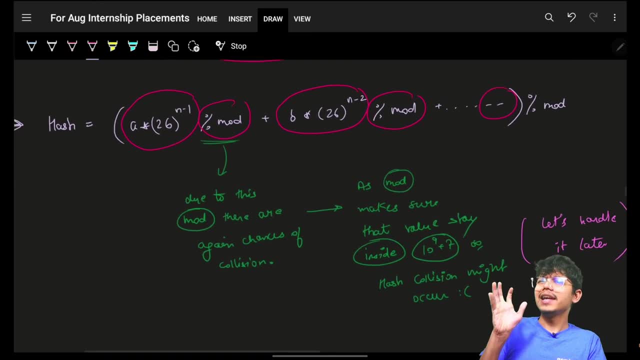 I know this value can go very large. I'll do a modulo. So I know, OK, I know I have to put my base as twenty six. I have to do a power, so I have to make a unique index. So I'll do a modulo just to be on the safe side that I always land onto my integer. 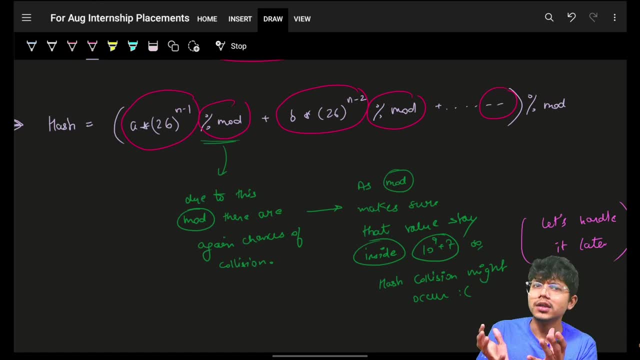 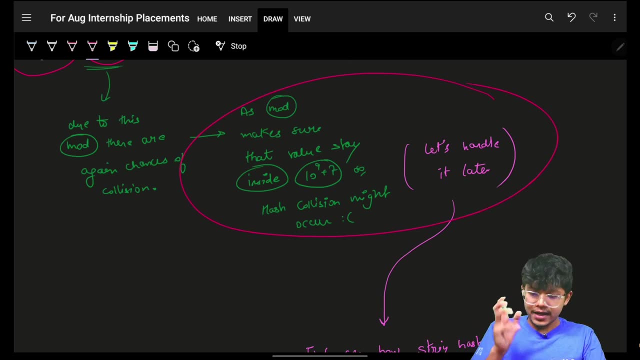 But, bro, you had a big value. You're reducing that value by doing a modulo. That's OK, But because of your modulo, still you can, because it's a very large value. OK, Very large value, large value, large value, and so on and so forth. 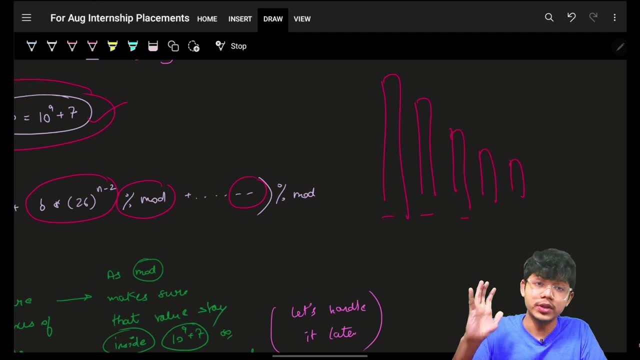 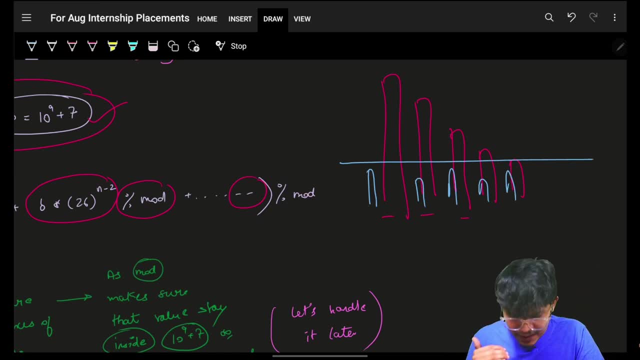 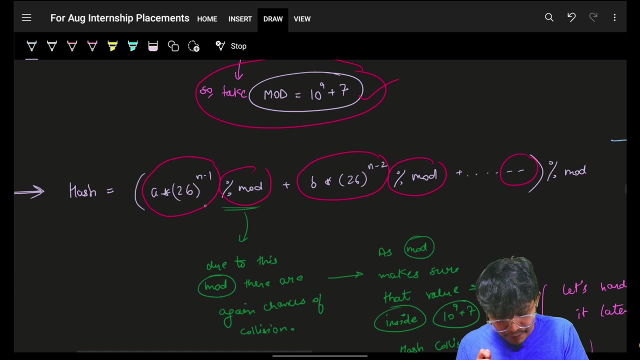 But you have made all the values small by doing a modulo. There can be a chance. after doing this modulo, you can still have your spurious hits, Which means you still might end up might end up having same, Which means after, after doing this modulo, you still again. that's going to be rare. 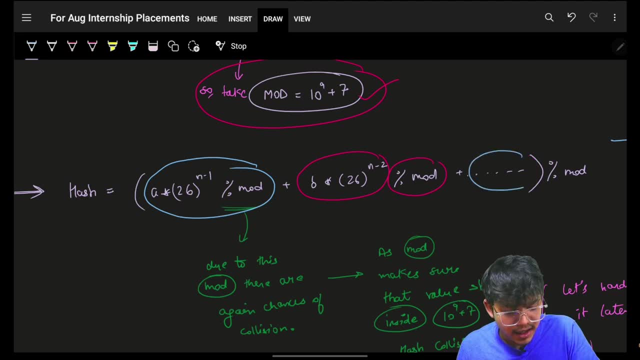 But still you might end up having this value same as some other mod value Earlier. if I would have not done mod, it would have never had a spurious hits at all. But I know it's not possible to have a very large value. 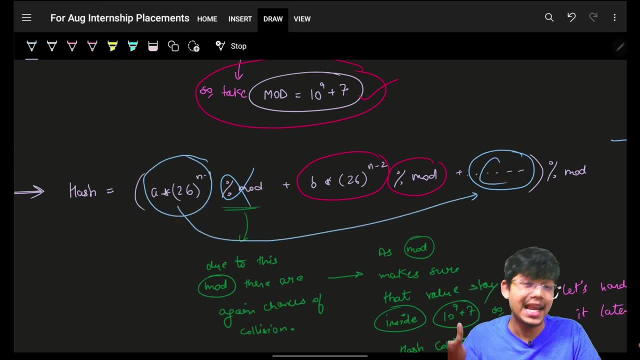 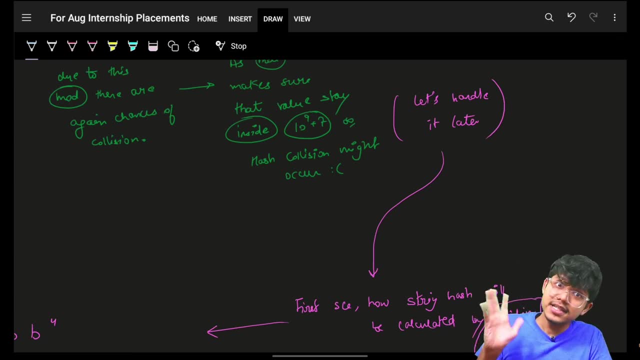 I have a boom mod for sure, So I will be having same. I can have same. That's a big thing, But yeah, you don't have to worry about it because, again, that's a very rare case. So it can be a case, but it's a rare case. 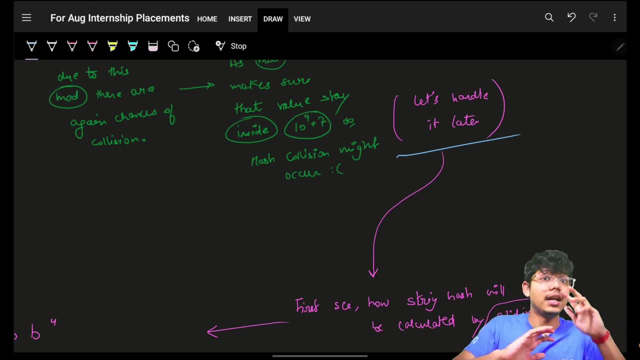 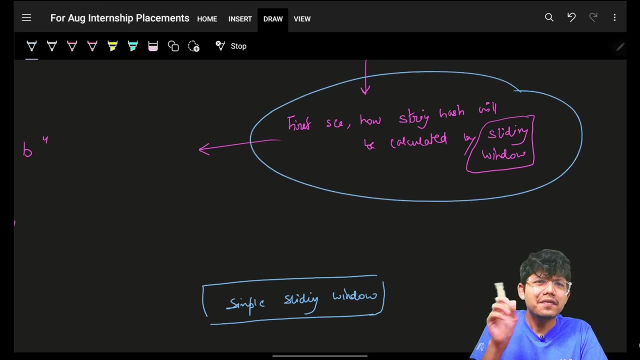 So we'll handle it later on by learning something else. But no worries, Hold on. So so far we have seen that we can do a simple sliding window to find the hash. But we saw sliding window by doing a simple hash for some values, just simple numeric. 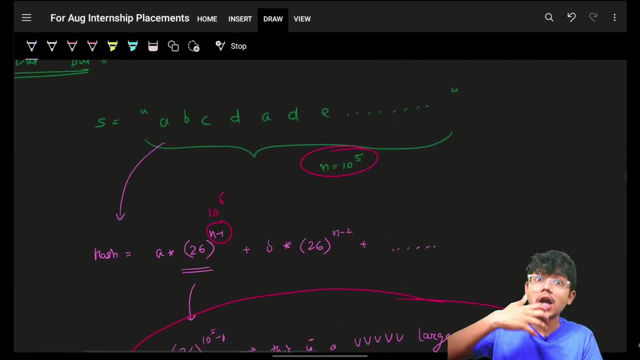 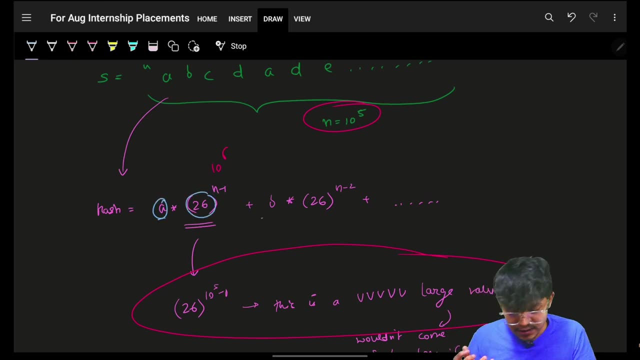 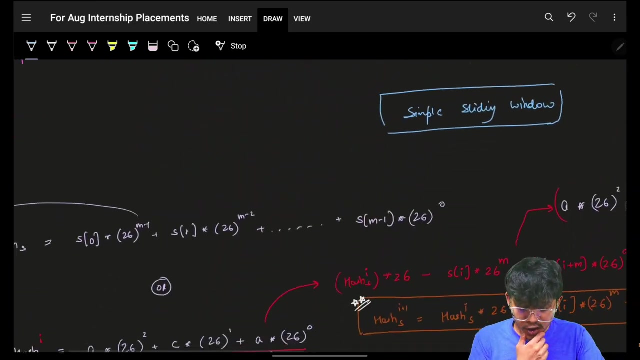 But now my hash function have evolved a lot Now. earlier my hash function was A, B, C, But now my hash function is A, So I have some radix again. This value is called as a radix, with some radix, its exponent, which is index, and then so on and so forth. 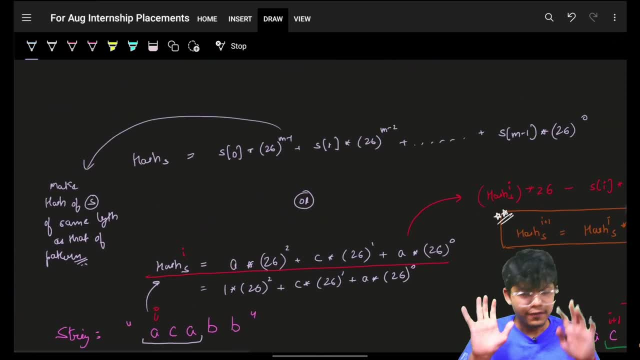 OK, now let's see how our hash function will look like. Again, we saw it will look like like OK character, which is S of zero. S is the string index of zero. Then radix, for us, which is 26,, which we have taken because we know it's. we can take anything more than equal to 26.. 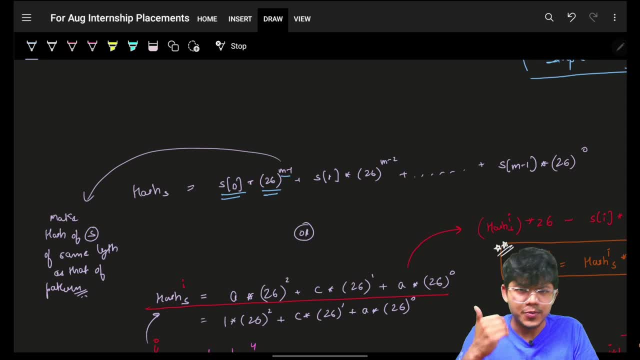 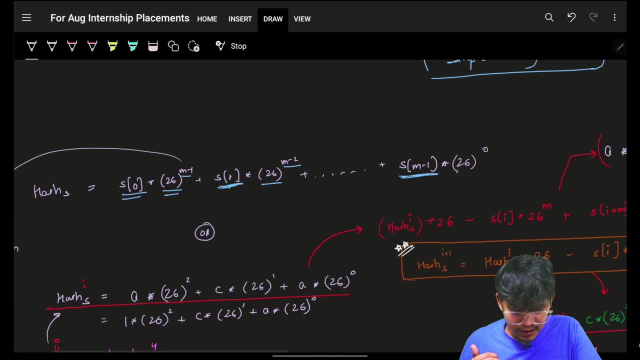 Now, Now Minus one, which means indexing, and then so on and so forth. OK, next character radix is to our index, and so on and so forth. Last character radix and its index: Like considering we are, we have the index from there itself. 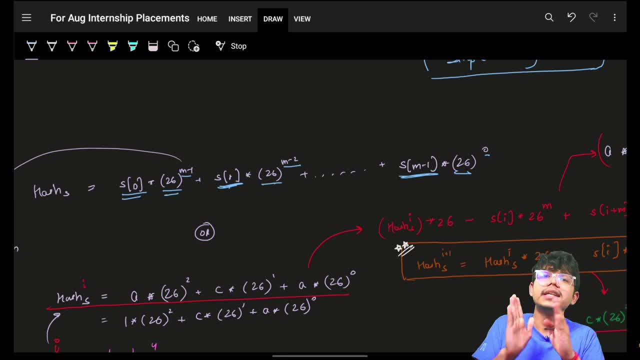 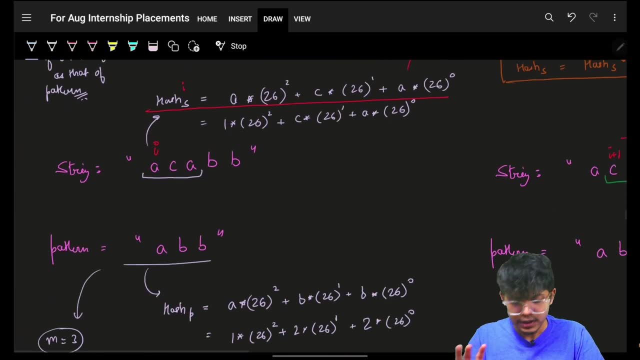 Again. you can also go in from left with the index as this, but then you have to modify accordingly. So now this is the rough formula for a hash which should look like. So let's see how we'll make again. We'll make the entire hash back, for both string and pattern. 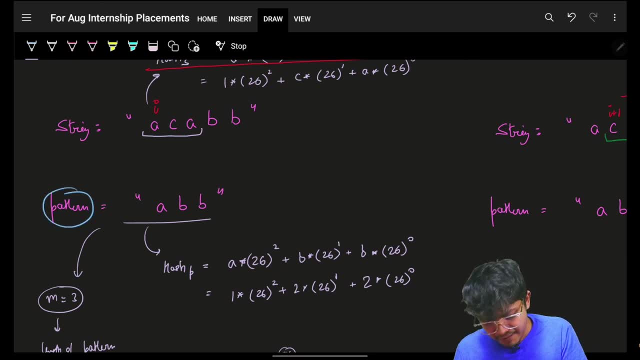 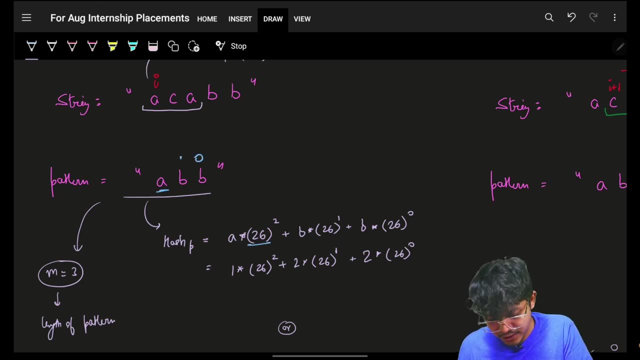 OK, so we saw one thing: that we have this pattern. Let's make a hash for it. So how should look something like: OK, we have a multiply by 26.. We know that index is zero, one two, So 26 is the ratio of two plus B. 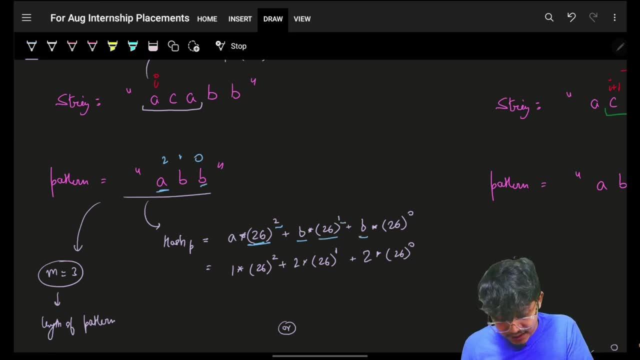 multiply by 26, ratio of one plus plus other character, which is B, by 26, ratio of zero. So now we have got this hash. OK, great, Same way, same way. I will compute the hash for my string as main string. 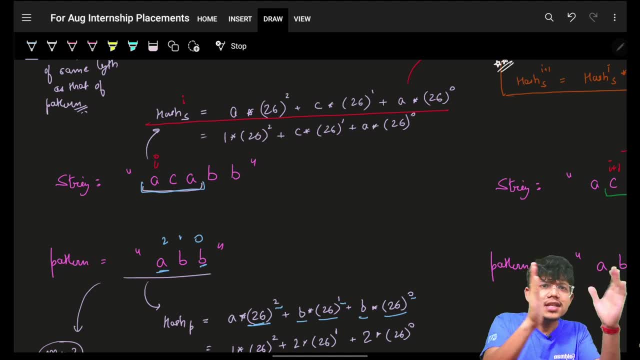 Again for the starting end characters, And then I'll use my sliding window approach for the initial M characters. Again, M is this size and is this size. So for initial M characters I'll use and compute my hash, But then after, after, onwards I will use sliding window, sliding window and so on and so forth. 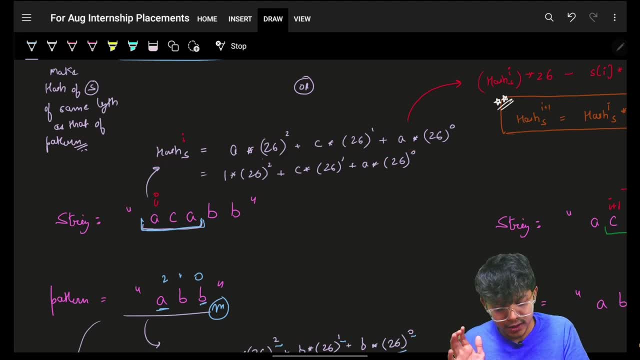 So for the initial hash, I'll just simply say: A multiplied by 26, ratio of two, again considering it is a zero, one and two. So A multiplied by 26,. ratio of two plus C: 26, ratio of one plus A. again A multiplied by 26, ratio of zero. 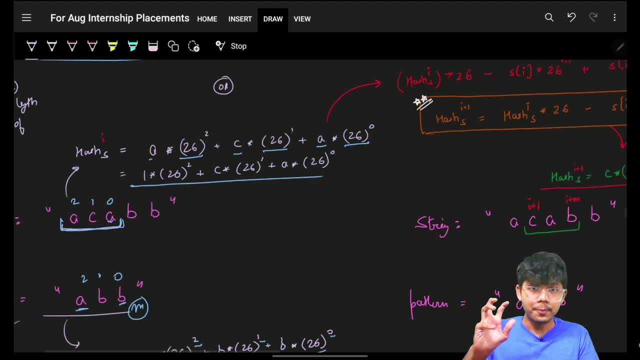 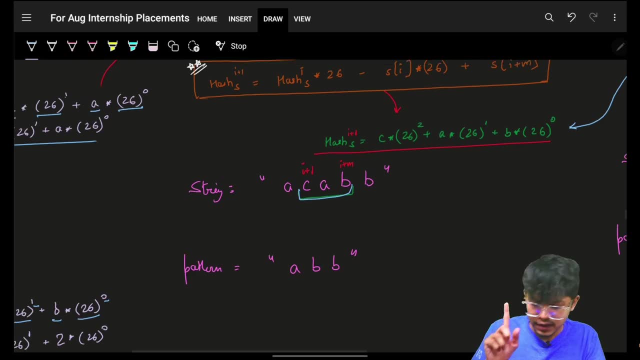 OK, we have done this. we have done this part Now. now comes the fact that we have to compute the next hash Again, although we will use the sliding window here itself, which means- which means what we will do again- first see how this hash- new hash- will look like. 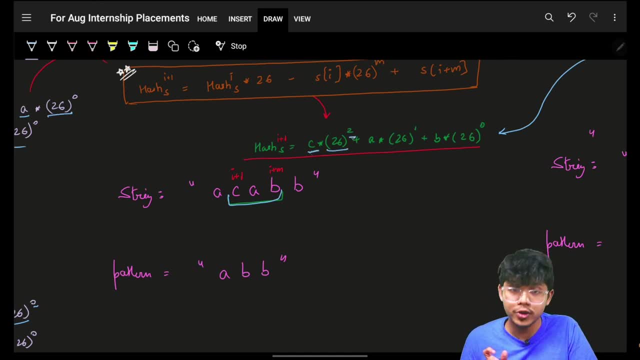 The new hash will look like 26,. sorry, C into 26,. ratio of two, Again, considering it is a zero one, two. like this, Then again: A into 26,. ratio of one plus B into 26,. ratio of zero. 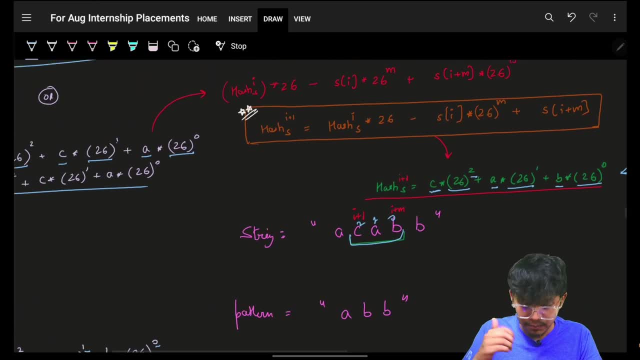 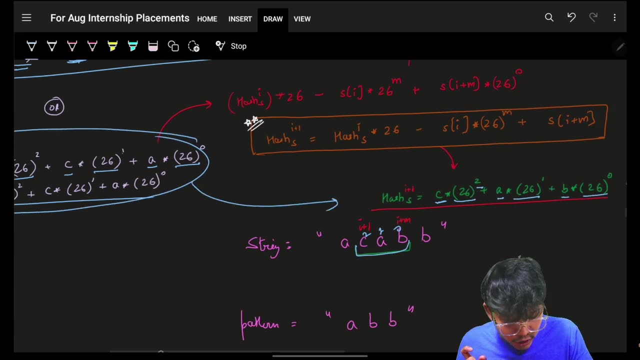 This is how our hashes are looking like, But my main task was I use a sliding window, which means I should actually use the existing hash and then I should be able to use and reach to my new hash, which is this hash. what operation I should do here? 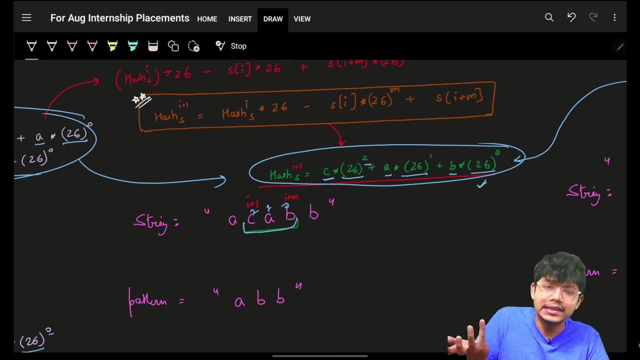 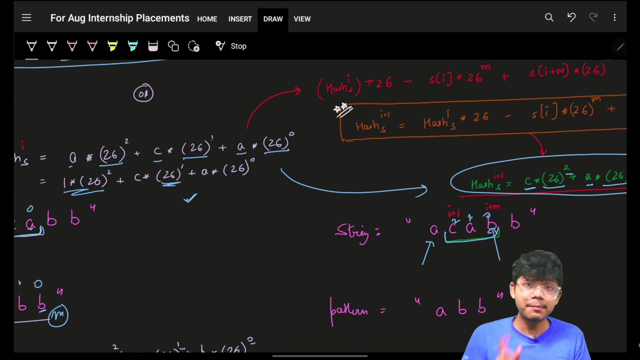 So as to reach here. we know, I'll simply add, I know I'll simply add a, B and subtract A, But you have to also make sure that you are actually maintaining this power also. So I had this hash in this: C is having one power, one power of 26.. 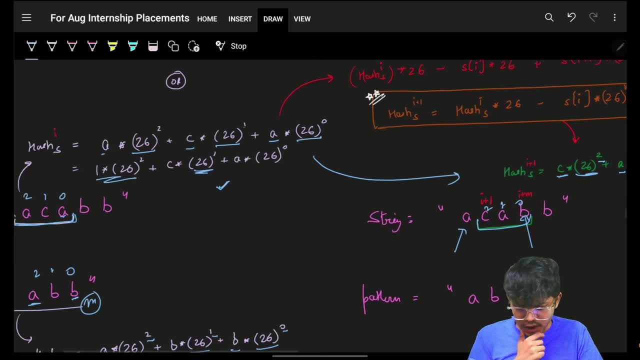 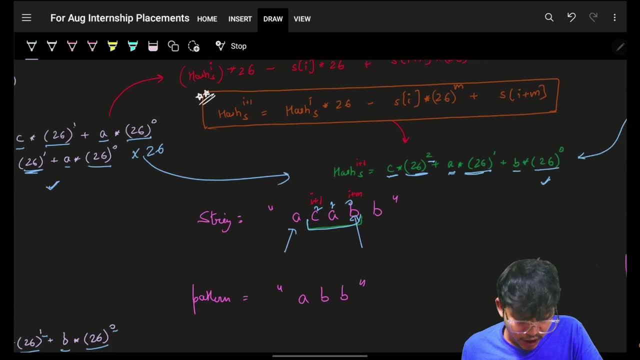 I can see C is having 26,, which is a full two. So I know I have to multiply by 26 in the entire thing, because A also has 26,. ratio of zero. A has 26,. ratio of one. So I know one thing: I have to multiply this entire existing hash with 26.. 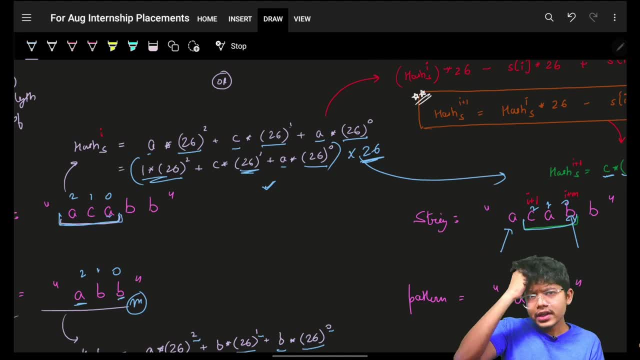 That's fine. OK, that's fine. But then I also realize that if I multiply that by 26,, that's OK. So all this will be, all this will become a two. OK, this will become a two, This will become a one and this will also become a three. 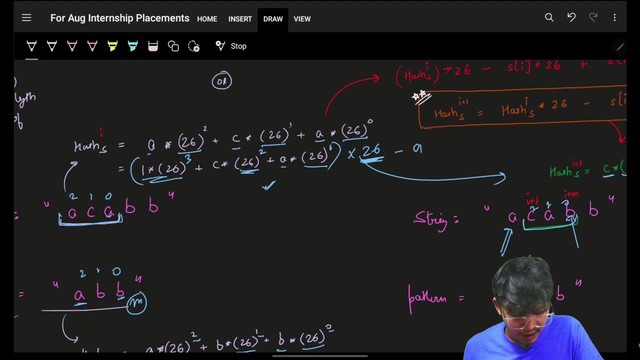 Then I have to subtract my A, because I know I have to subtract my A. But subtract my A by what power? I have to multiply with 26 hash power, what It has become a three. Now I, if you remember, I had put indexing zero one, two, indexing was two. 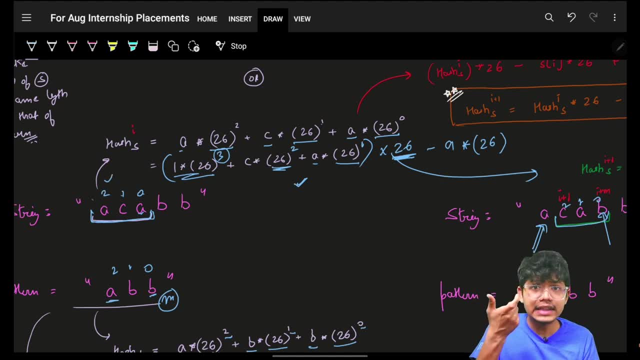 which means I had three elements. that's the reason indexing was two in the last. So I know it has become last index plus one, which is nothing. But if it is zero then it can go to M minus one. So it become M minus one plus one. 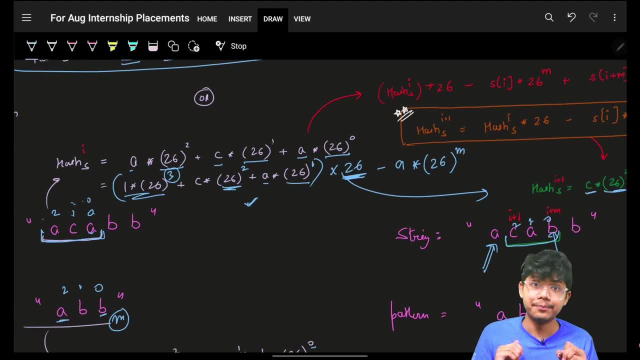 So it became M. So I know I have to do it And this is for M in that. OK, this element is gone. But I have to add this element which is last element, which is nothing but B. So I'll add a B, But again, add a B with what? 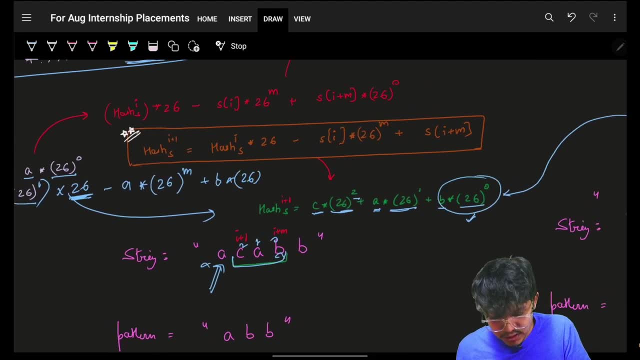 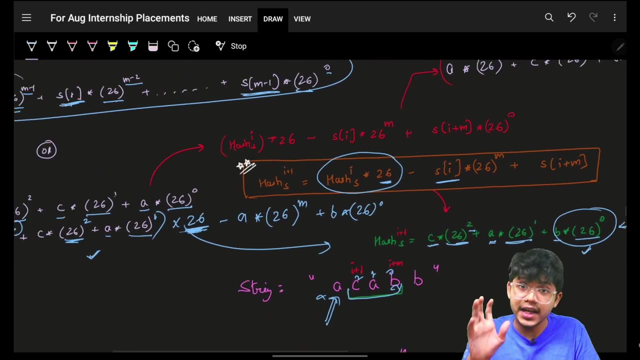 B multiplied by 26,. ratio of zero. So I multiply by 26,, ratio of zero. So that's how, from my existing hash, I'll multiply by 26.. Subtract my S of I, again considering, although considering my I is here itself. 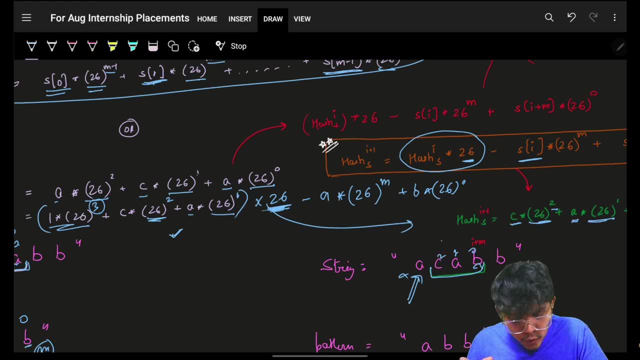 Again, when I show you the code, my I will actually would have moved on, So I would have been here. So I will be actually referencing with I minus one, But right now, again, that's a small change which you can go anyway, here and here and there. 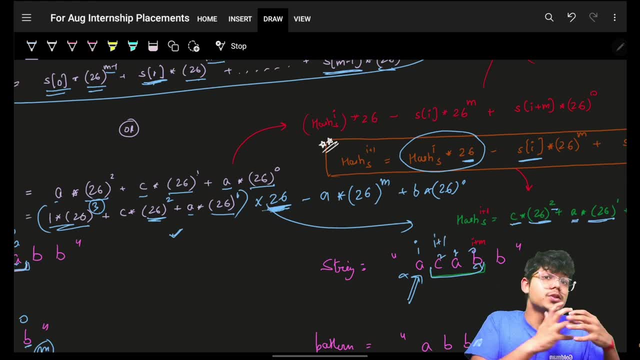 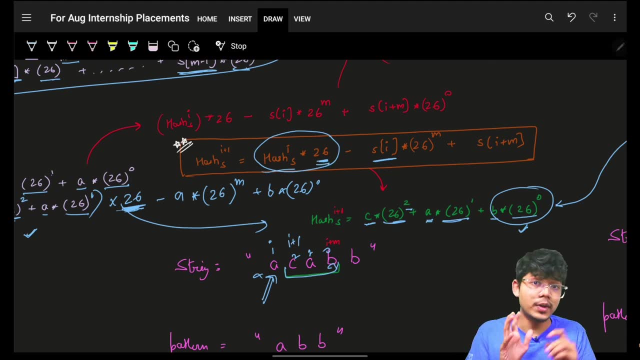 So right now, considering my I is here itself, I am trying for I plus one hash, which is the next hash I'm just trying for right now itself. Then I will say: I'll take the existing hash, multiply that by 26.. 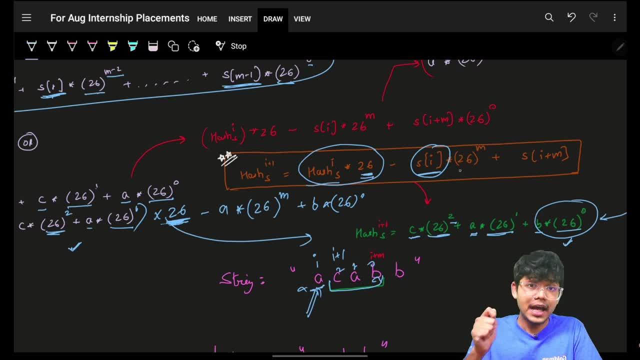 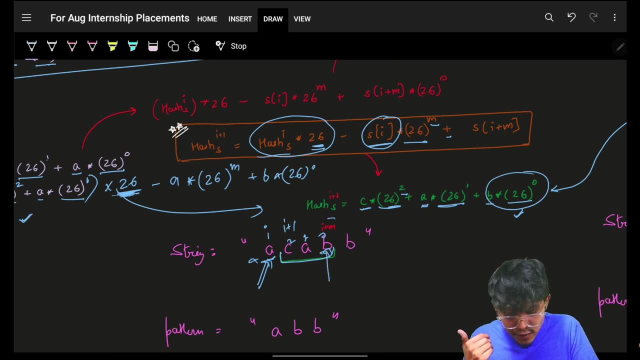 Then my existing index value, which is A. right now I multiply by 26 hash power, M, And then I will simply add up this new upcoming vector, which is S of I plus M. If my I was here, then I plus M will be here. 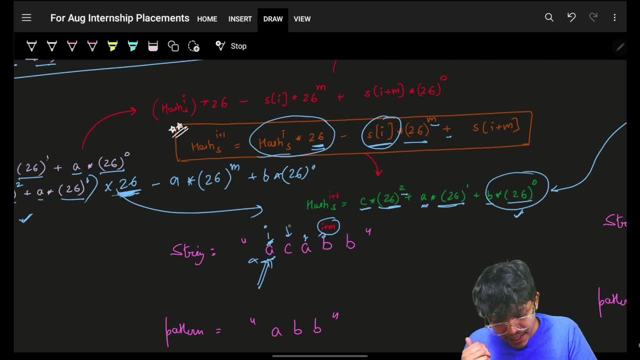 Remember in the code. remember in the code when I show you my I will actually be here Again. you can also keep your I here itself, But then so this index will be I plus M minus one. So keep it here and there. 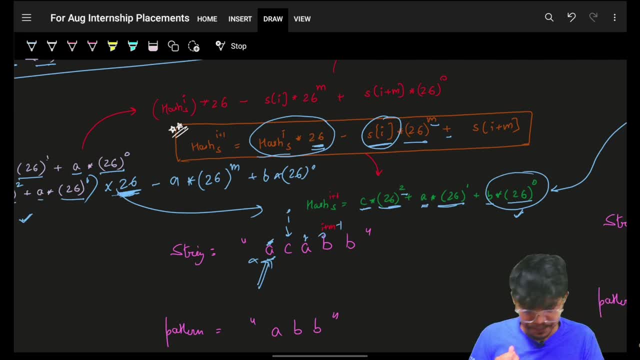 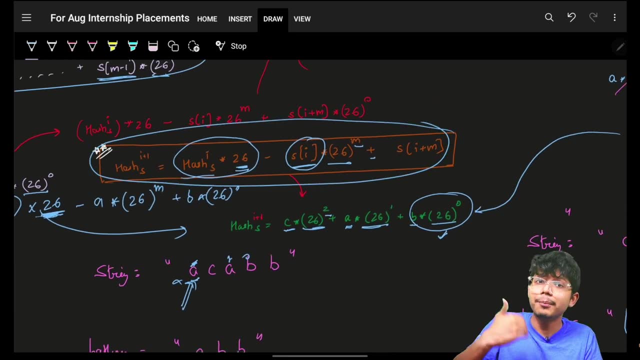 Anything can go. It's just logic building. Problem solving is more important. Now, coming on back, we will get a new hash. So this is how I can simply, in O of one operation can compute a new hash. So that's again. I can repeat this exact same process to get a new hash for the new string onwards. 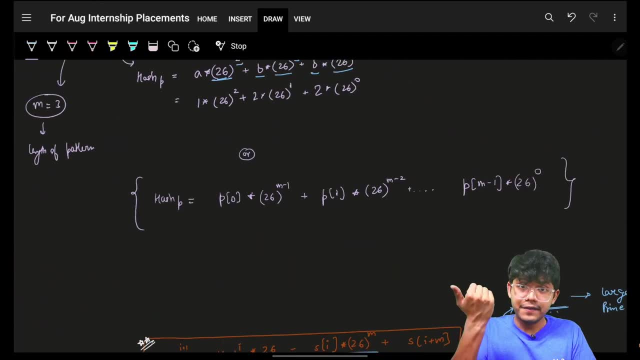 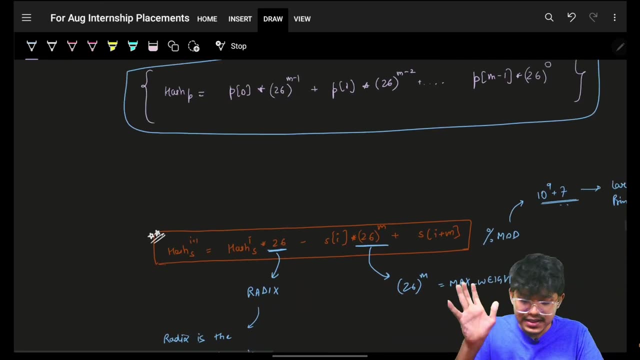 Simple sliding window. So now we have seen that we will find the hash of the pattern, that will look simply, of how we would simply go and find the pattern hash And the same way I can keep on finding my new hash. Remember that's a hash. 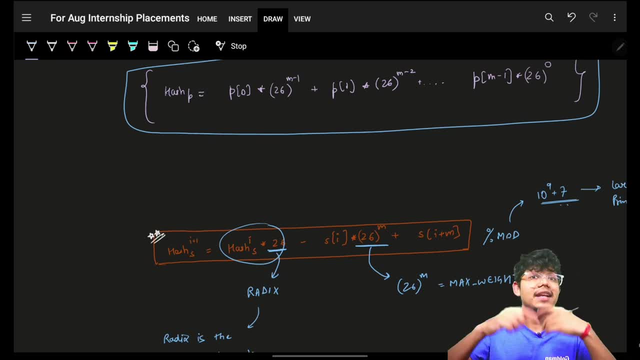 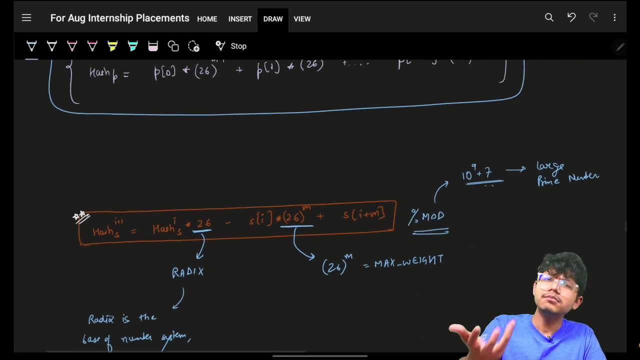 But make sure to do modulo at every step because the number it will end up becoming very large and you cannot store that large number. So please do the mod with a big prime number. We know the standard big prime number is one in nine percent. 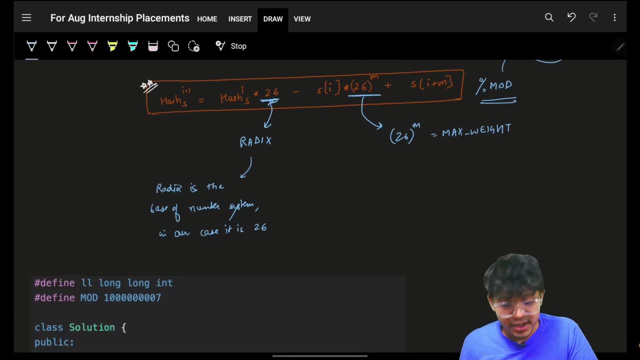 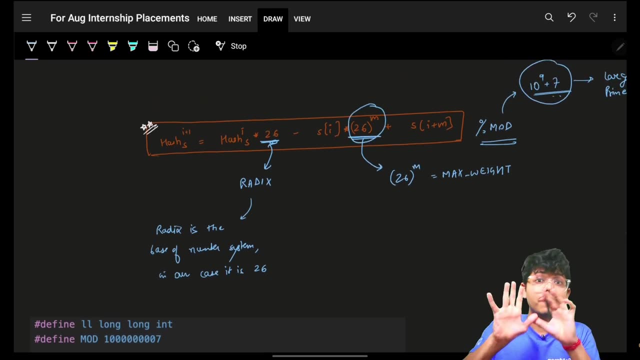 Cool. And again I have told you that this number is called as a radix And we were just doing again in the code set. You will see that this value will remain always constant because I am comparing the sliding window of size M, So this will always remain constant. 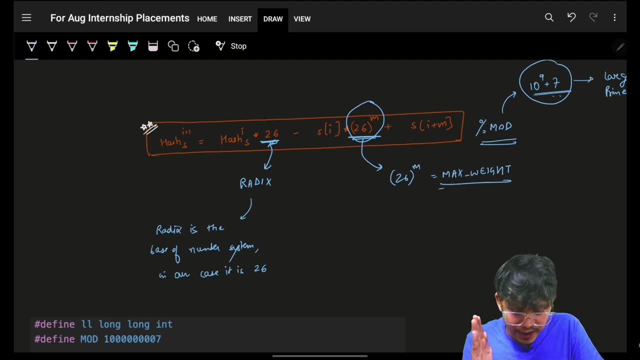 So I will put it as a variable which is called as a max weight for my code, And then, in that I'll using, I'll be using this actual. I'll firstly compute this value, because I know I have to compute this value with doing a mod itself. 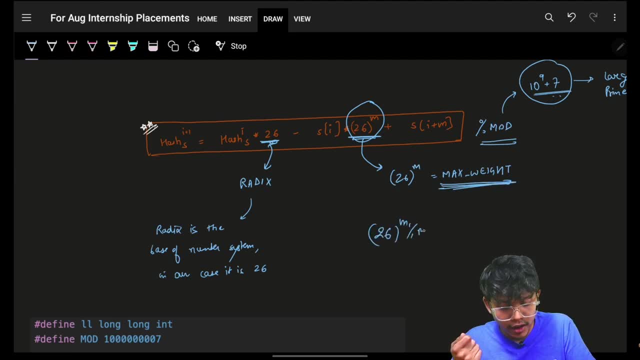 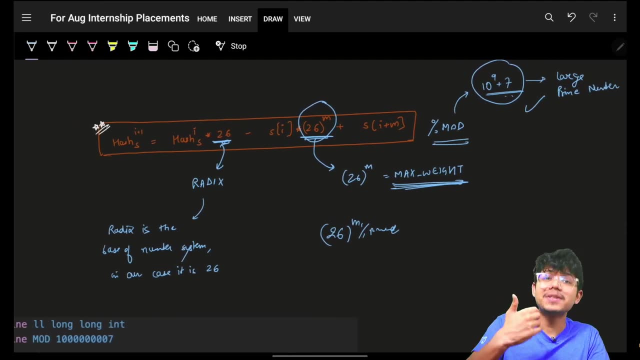 So this max weight will be twenty six ratio over M mod with the mod value. Now mod value is one nine percent. Again, everything will be mod. But it says that I will show explicitly that, OK, what things are actually being mod at that specific time. but everything will be more every time. 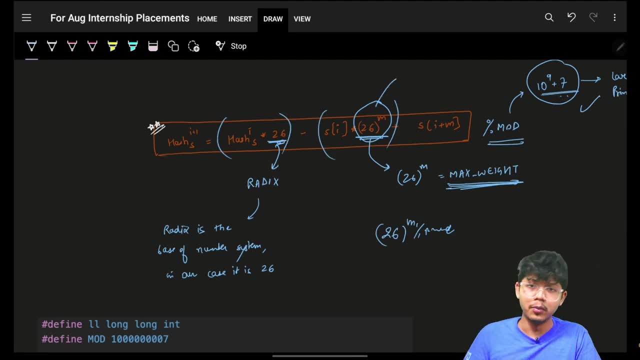 which means this will also be more, This will be more, This individual will be more. So everything needs to be in the mod range, which means in the integer range. now, and you know that you will simply can add S of I plus M, multiplied by twenty six to zero, which is nothing but one itself. 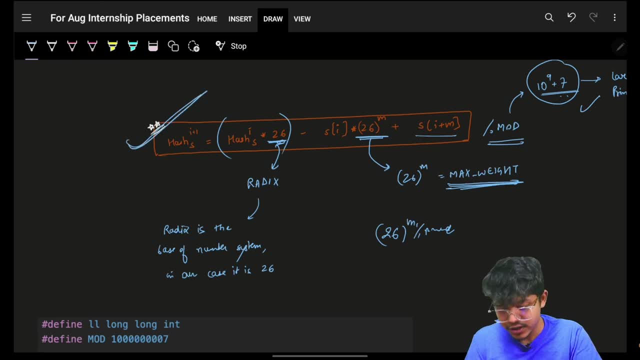 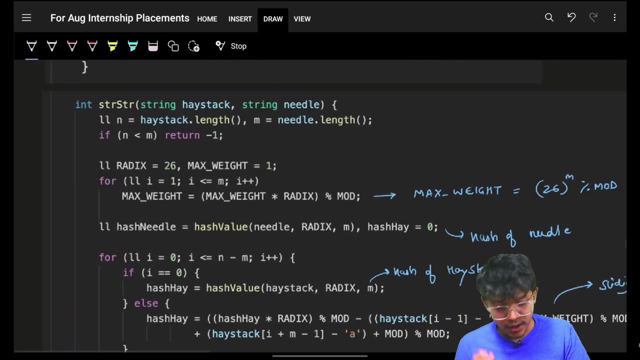 So multiply by one. It doesn't matter if you put it there or not. That's how you can simply keep on building your hash. Let's see the code again. That's simple string comparison code. So firstly, if you remember what you are given to task, find if this middle is inside your stack. 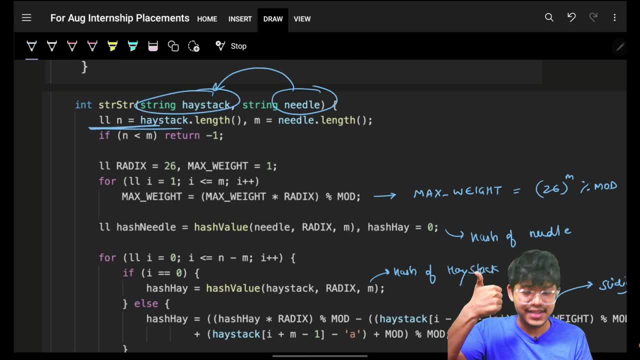 Now, if your needle size, let's say your stack size, again he said it was a big array, Needle was a small array of size and of size. And first basic thing is: if, what? if you're M, which means the needle needle string is itself way big, and for sure it's not. 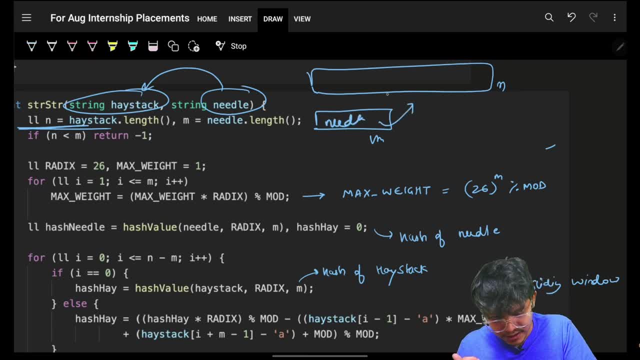 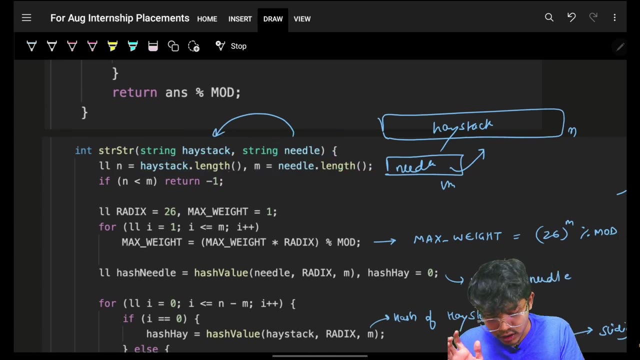 possible to find your needle in the stack. So this is needle and this is history. Same needle needle stack. That's how he stuck. Now I can simply go and check the cable. It's still. it's his stack. Now, if you're, his stack is itself less than zero in time. 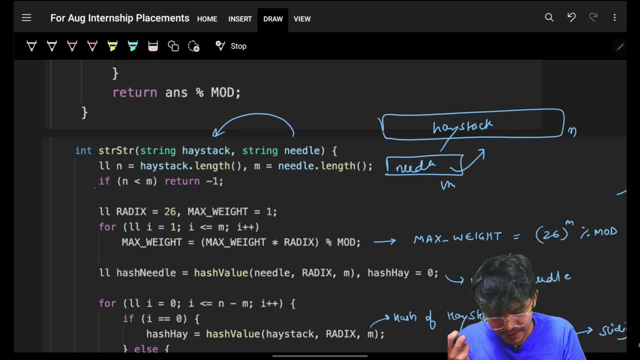 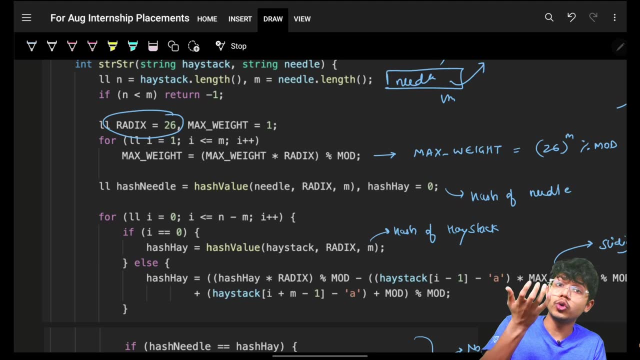 it's not even possible to find anything in his stack. Simply put it on my side here itself. Now let's go and start off. Firstly, if you remember, my critics will be nothing but twenty six, and then I have to find my max weight max. 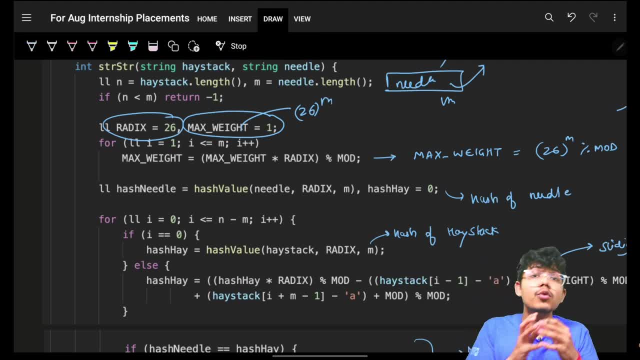 But, if you remember, it is twenty six And so I compute that max Weight so that I can use that everywhere. I don't have to come back again and again. I'll simply compute this and keep on using that. So I'll simply know it is twenty six multiplied by any time and times and times. 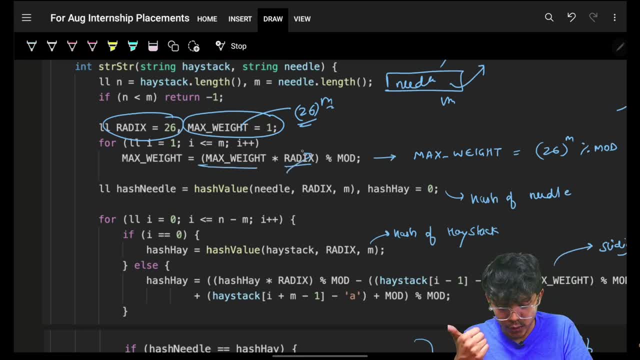 So I'll simply say max weight multiplied by which is twenty six for us, As you can see, M times it is being multiplied, The loop of M. here is a loop of M And that's how I compute my max weight, which is being being my model itself. 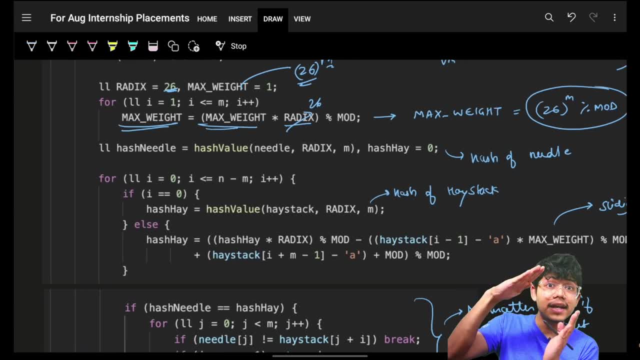 Now, when this max weight is done? now your next task was compared. So you have to find the hashes of your string M string of length M in your haystack versus your needle hash. So you have to find the hash of needle. So I will find the hash again. 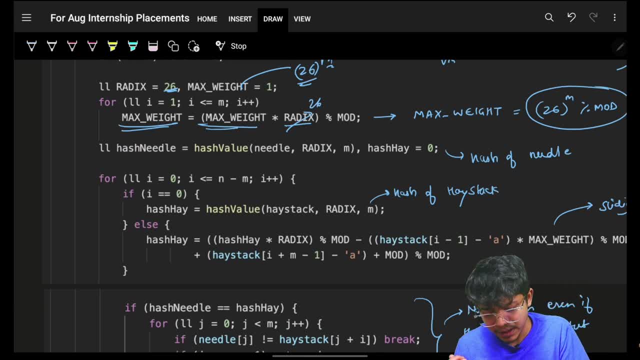 This hash will be an integer value, But to be on the safe side, I always keep a long long with me, Although it will always be an integer limit, But still to be like. maybe some way some value becomes a bit more. 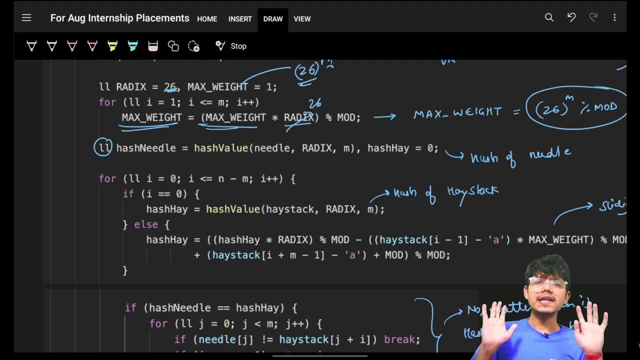 And then it is being multiplied by something, something, So that, to be on the safe side, I always usually keep a longer And I also recommend a contest and stuff. Please keep a long, long, So as to be Like conservative that OK, things are going right in your direction. 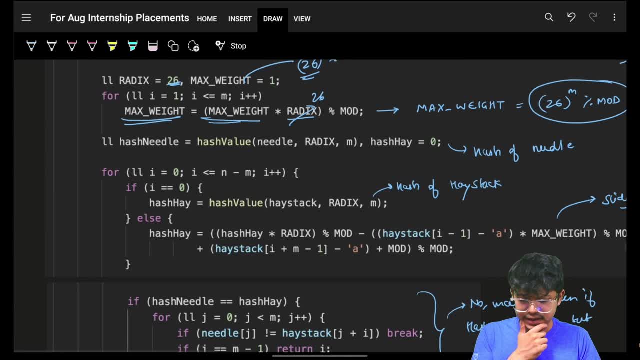 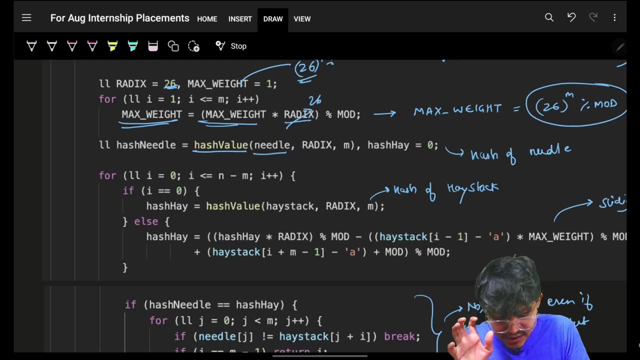 Now, coming on back, not what we can do is that you simply firstly find the hash value of a needle. Again, I will say: this is the needle string for me, This is the radius, which is, which is, which is right on twenty six. 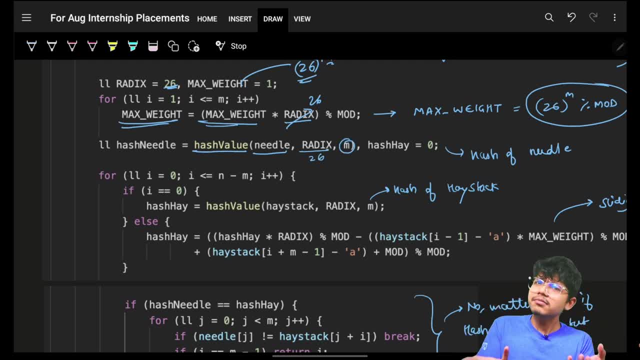 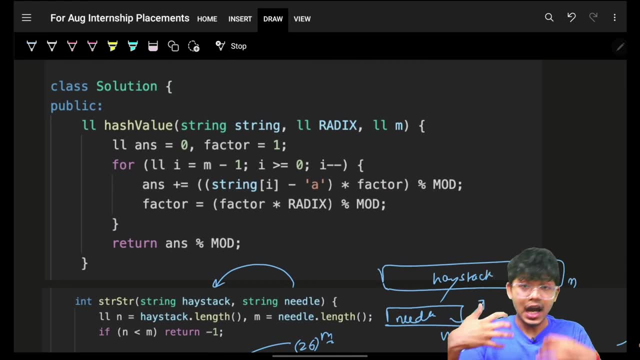 And the size of my string, which is M, length, M, And then I will The hash again. this hash is the hash function which will ask you for the string. Now, if you had remembered, let's say, our string is needle. 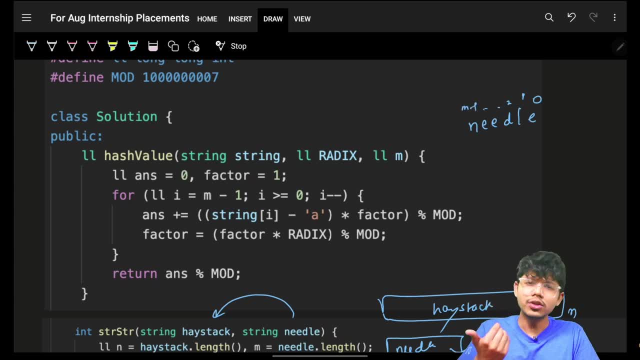 So it will go zero one, two up till M minus one. So again N into twenty six M minus one, plus E into twenty six M minus two. That's how the things will go, As you saw above. also saw the exact same stuff that I will go backwards. 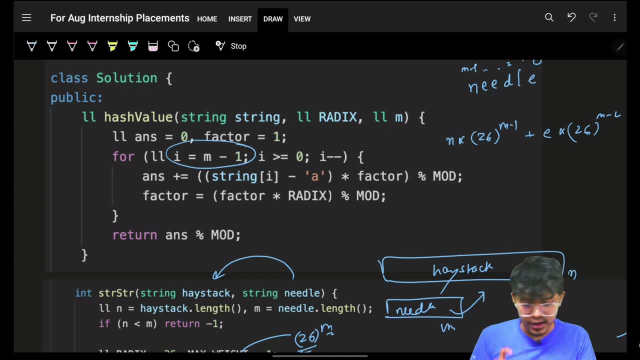 Backwards, which means, OK, my eye is going backwards, And then I'm Simply computing my answer- See string of I minus A multiplied by the factor- And then simply always remember to do a mod. So this factor is initially a one. 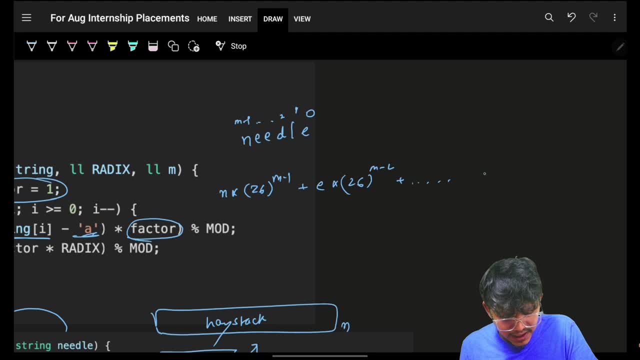 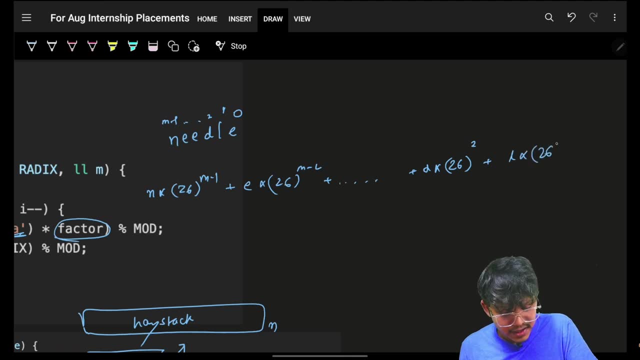 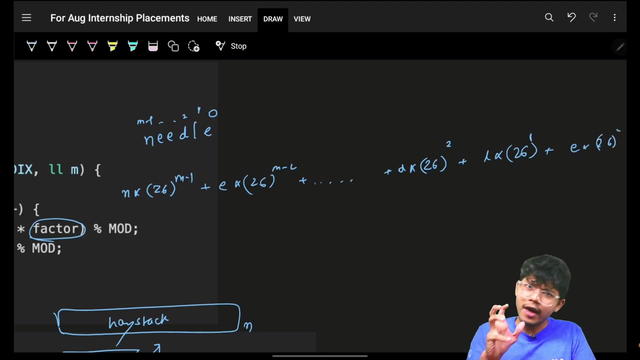 So what will happen is- I know I have to make something like D into twenty six, ratio to the power, two plus L into twenty six, ratio to the power of one plus E into twenty six, sorry, E into twenty six. Ratio, power zero. I don't have to make this. 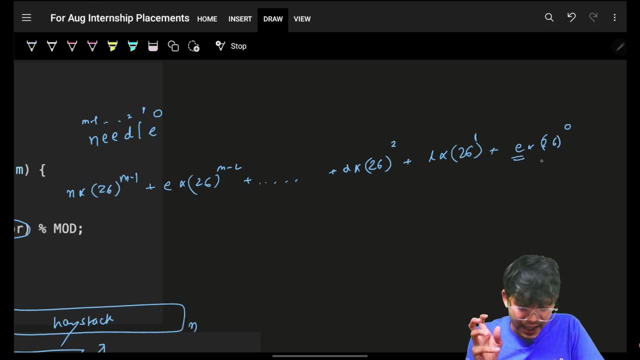 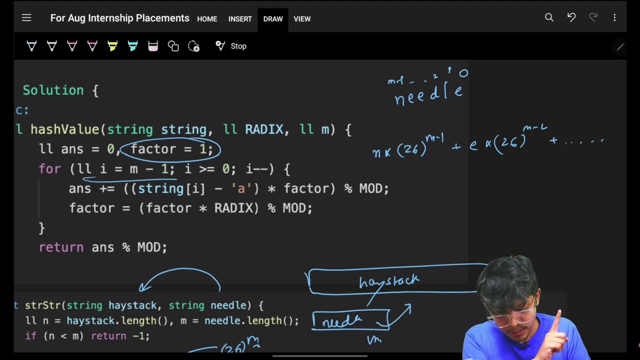 So I know that in the very beginning I have to put E and then twenty six ratio to the power zero. So I know in the beginning again, I'm going, I'm going in from the very end. So I'm firstly getting E itself and then 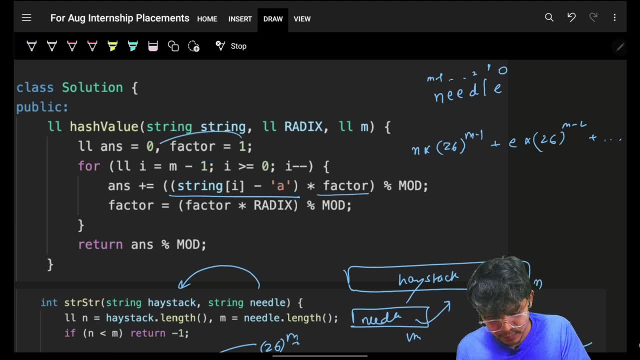 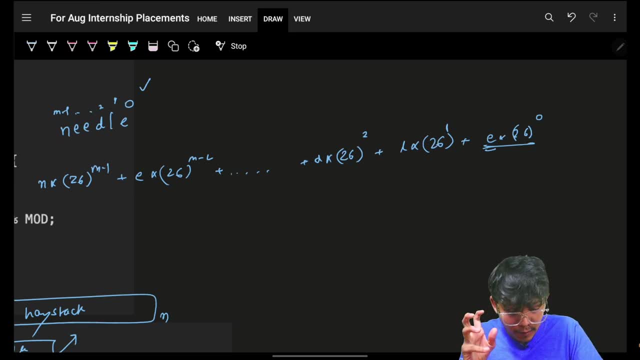 say: OK, E multiplied by factor. factor is initially a one for me, So I did a E multiplied by one Again. if you had remembered, I already told you that for my E the number is one, two, three, four, five. 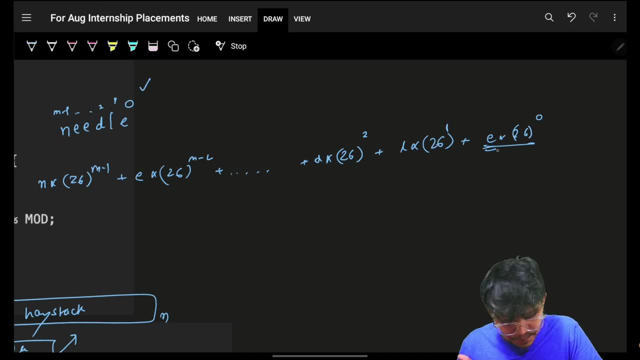 But I'm taking number as number, as four for E. So I'll just say E minus A, For example: see again: A minus A will be a zero, B minus A will be a one, C minus A will be a two. 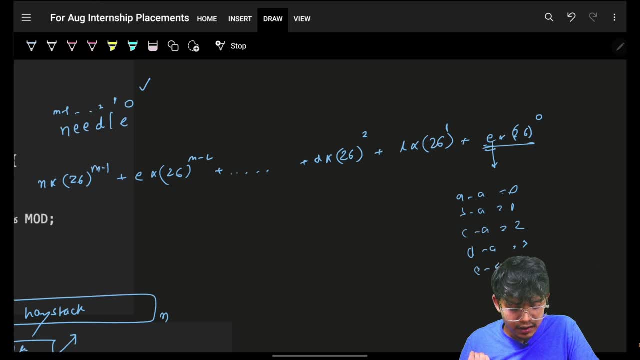 D minus A will be a three and E minus A will be a four. So that's the reason. I will say simple one thing. It can easily be said as four into twenty, six ratio to the power zero, which is four into one. Cool, OK, this is done. 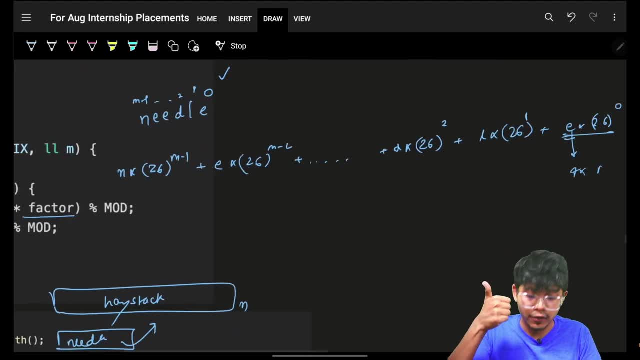 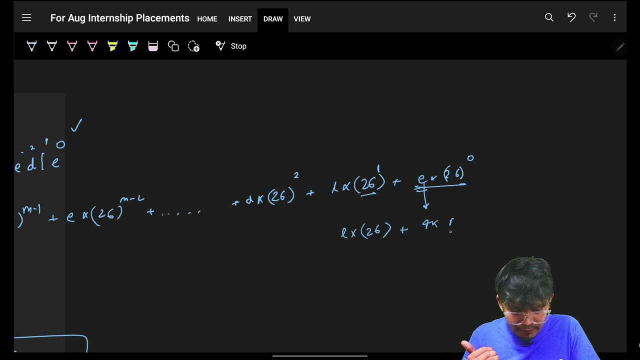 Then I will multiply my factor with the Radix value, which is twenty six, So as to the next value. So I'll just say L into twenty six, because I multiplied my factor with twenty six, and then D into factor, into Radix value. 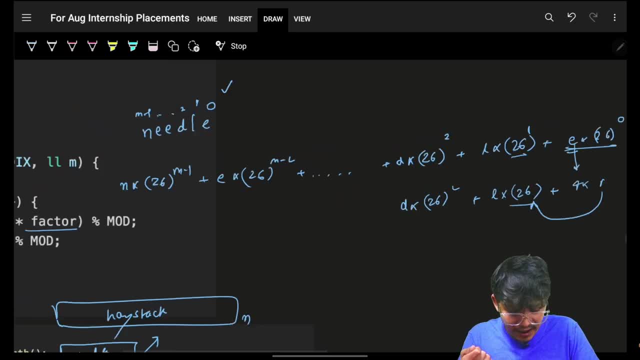 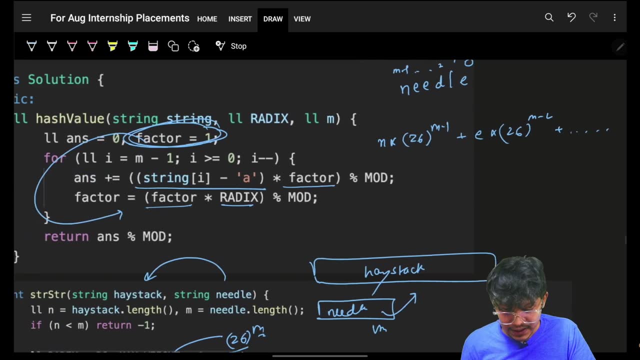 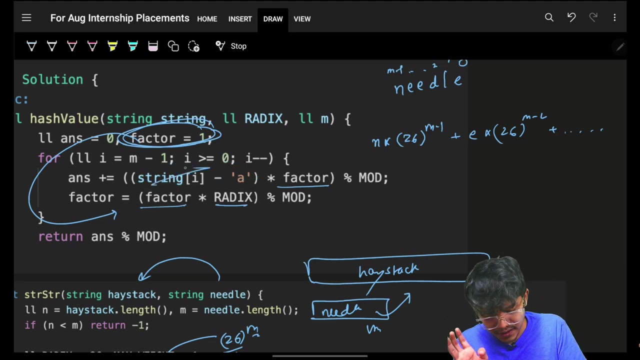 So I'll just say twenty six square. So this is this again. factor was just one. I'm keep on multiplying by Radix and I'm trying to build my answer from back itself Again, because of this reason, your A is value will be nothing but earlier if I put A here. so A minus A will be a zero. 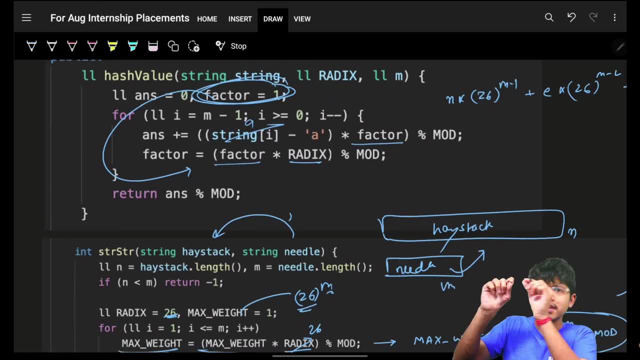 So, as in the code, we will see that we are mapping A to a one, then B to a two, But yeah, here A will map to zero, B will map to one, and so on and so forth. So because of this, I'll just simply scan, say this will actually how it will look like. 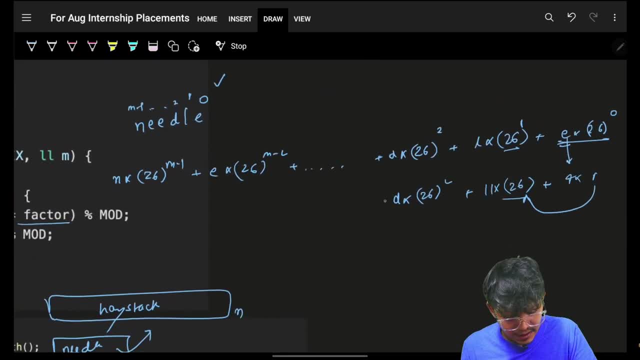 So I will have A. let's say L is twelve, right, So it will be eleven. D is four, so it will be three, and so on and so forth. So E will be four into twenty six. ratio to the power M. 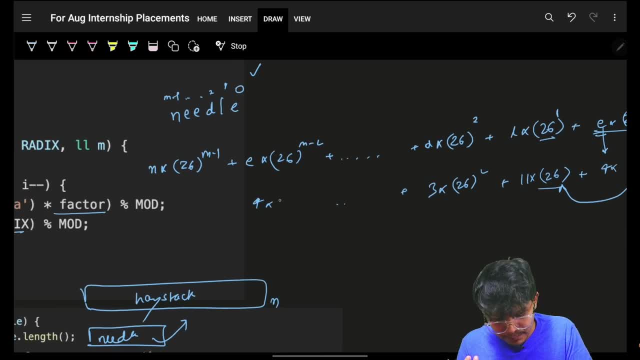 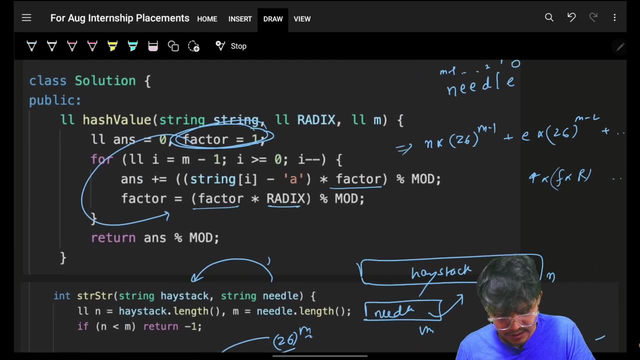 Minus two, and so on and so forth, But I'm multiplying my factor with the new Radix value, which is, let's say, R, And this is how I'm actually building my factor and then building my this entire string. OK, when this entire portion is done, 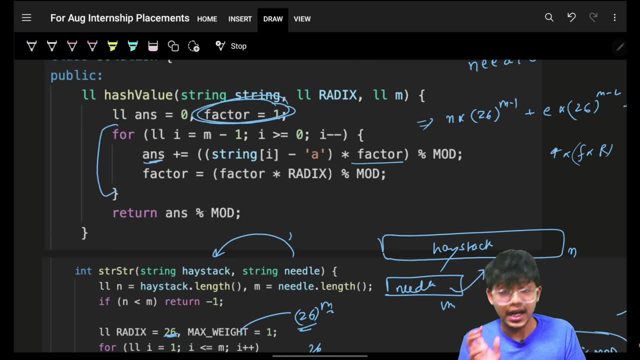 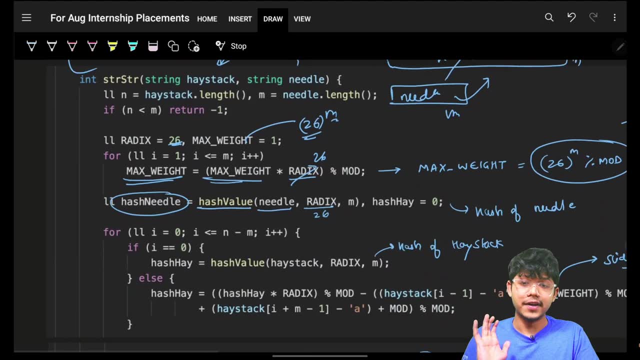 you will see that you will actually be having your actual answer. Answer is nothing but your hash. Again, please make sure to do mod at any step whatsoever. Now you have got the hash value. That's a function which you have got, OK, simply. now let's go on to the actual, actual string S, because now you have just 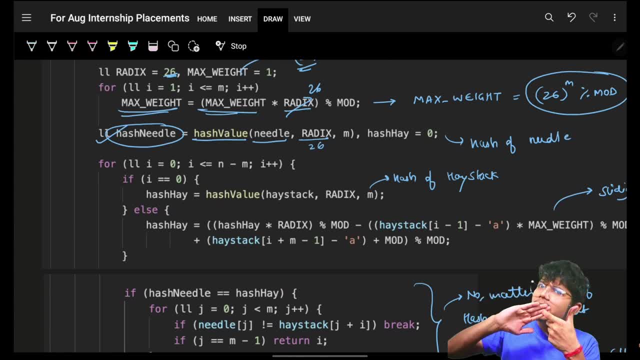 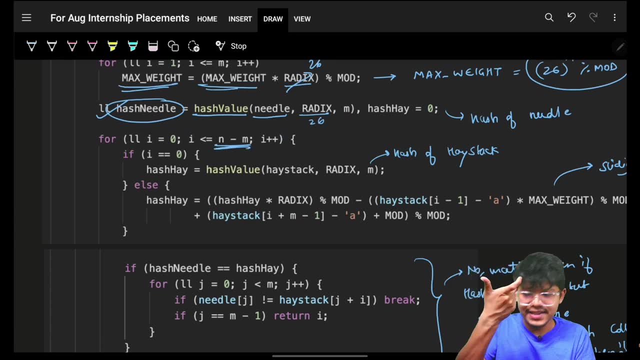 got the hash of the needle. but you have to find the occurrence in your main string, S. So go on to your actual main string, because you know the length of the pattern is M. So compare up till the N minus Mth index. 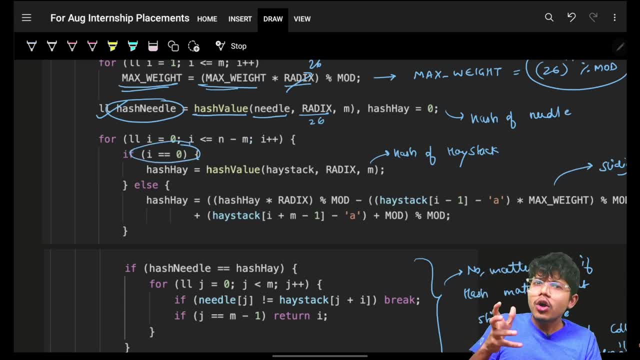 OK, in a very basic initial index you know you cannot do a window, You cannot do a window movement. in the very initial index You have to actually go on to the entire length M in your string of length N. So I'll find the. 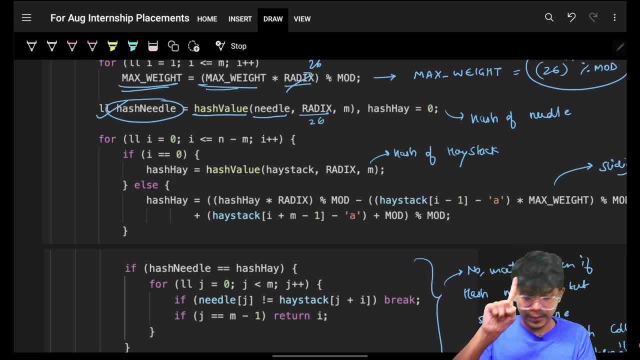 hash of Haystack. first time. only only one time. only one time. First time I find the hash of my Haystack. Again the same function. It will give me the hash value of my Haystack of length M and giving this with this as the radix value. 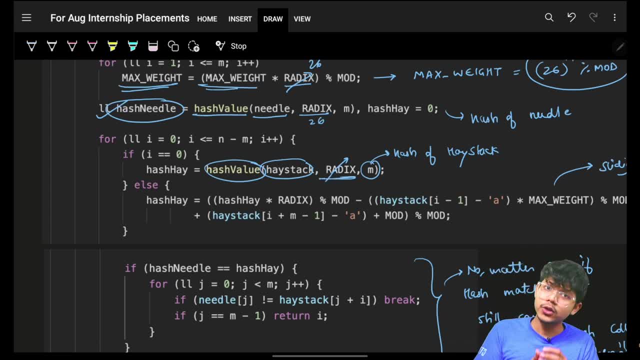 Now you might ask Aryan, this radix value is constant. for us, We will take it 26.. So why have you passed it as a function? No worries, you will see it later on why I have passed this as a function. 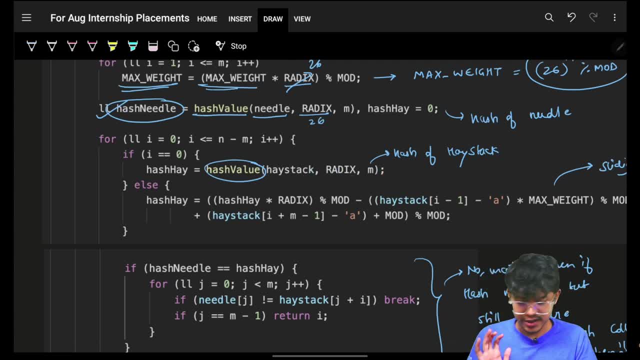 But yeah, right now, let's imagine that this is constant for us. So now you have got the first hash value of Haystack. OK, now, as the index will move in now I simply use a sliding window, As I said, existing hash value multiplied by 26 and existing like go on to the index. 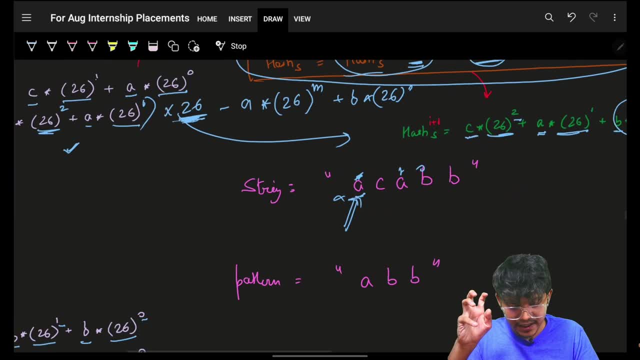 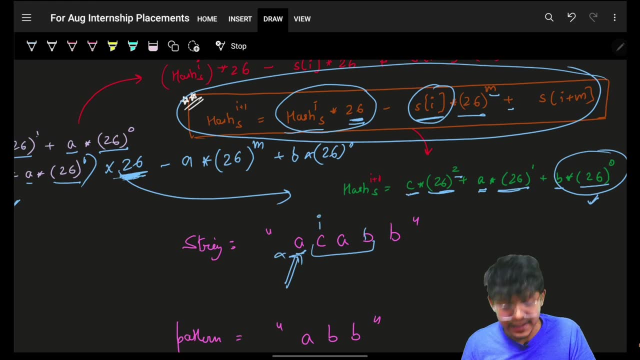 Again. if you had forgotten, I had told you that if I am moving in my indexes, So if you had forgotten, if this is gone, yeah, if this is my current window, So my I is here, I minus one. I have to remove. 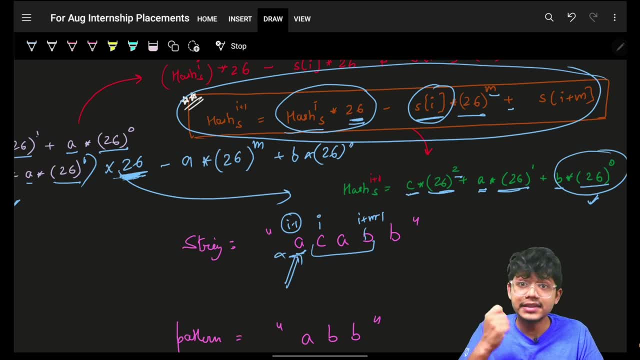 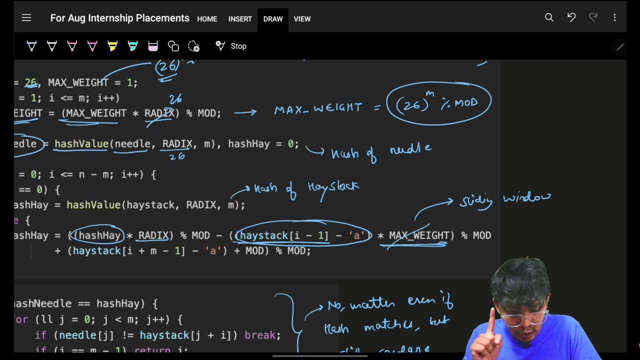 And I plus M minus one. I have to add in the existing window. So exact same stuff. I'll do, I minus one index. I have to remove and again removing. I have to do a 26 ratio, power M, and then I plus M minus one. 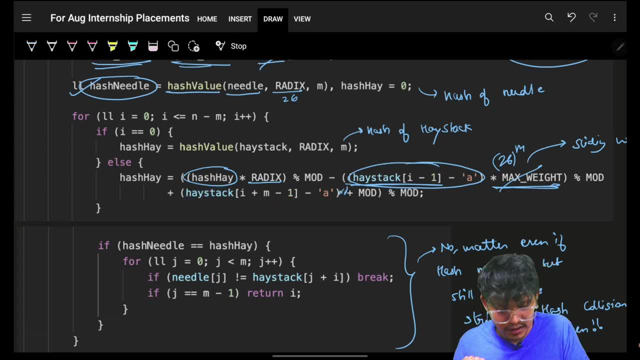 I have to add back. So again, multiplied by, multiplied by one one. No, worries, don't write it at all. This is, this is I am subtracting, which is this hash value: I minus one. And this is I am adding, which is the new upcoming character. 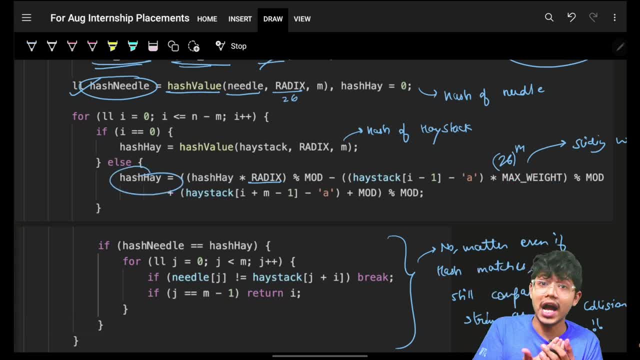 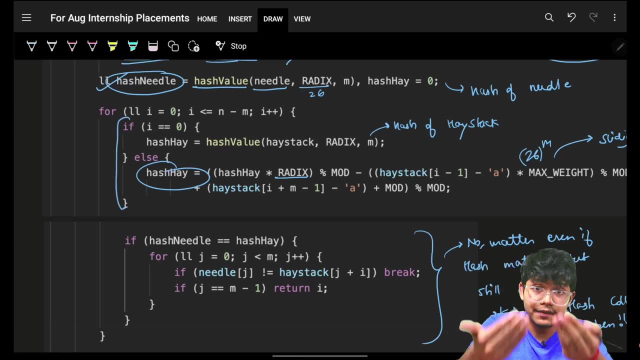 And that's how I can simply get by using the exciting window, the new hash of the window. Now, when you have compared a specific, when you have built the hashes- no matter if you had used a sliding window or if you had completed for the very beginning time, when the hashes have been completed, 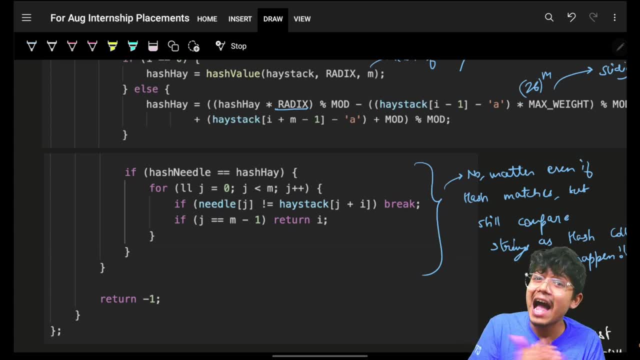 Now I told you there can be a chance that you can still have a spurious heads. So you will still, even if, again, if- your hashes has become equal, still I will go and actually compare both these strings. Still I'll actually compare both the strings again. 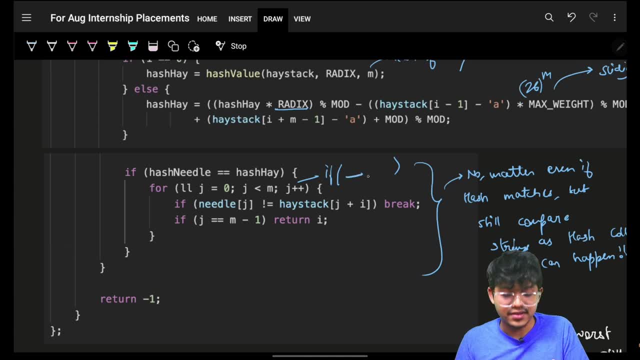 I can simply write it as a simple condition If my this substring is equal to the actual needle string. But yeah, I just told you that, how you can actually see that again, I'm actually comparing the strings. Even if my hashes be matching, I'll still. I'm still comparing my hash of that. 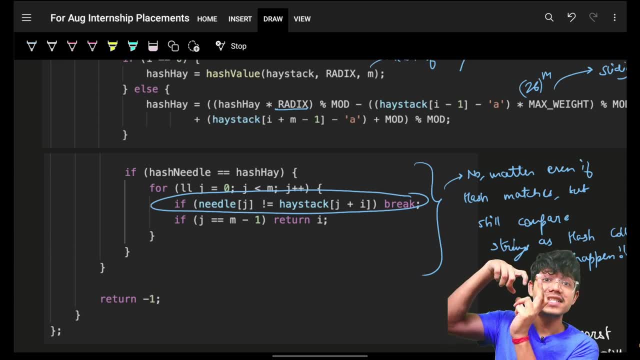 specific string of length M of my string pattern, of my string S, which is the haystack with my string needle. I'm still comparing That specific thing again, if I cannot find something, if I say, OK, that's, characters are actually matching. matching for us, bro. 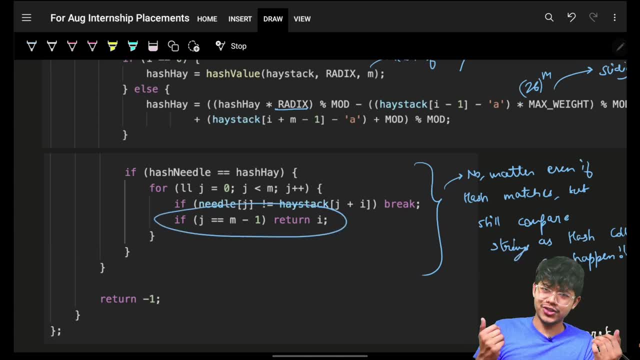 But if it is not, bro, you have got the match. You have got the match, bro. Simply return, simply return. So I know that if I have got both actually matching, simply return that specific index, because that's the first occurrence of our match. 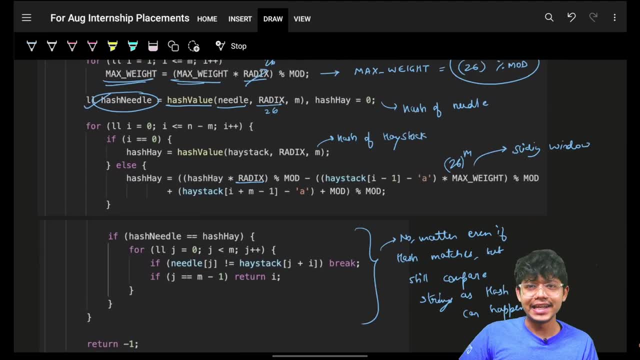 But you will say: Aryan, you did so much of headache and now you are saying that it is exactly same as having a single simple hash function. What's the point? You wasted our 30 minutes. No, bro, This hash collision which we saw here, it will be very less. 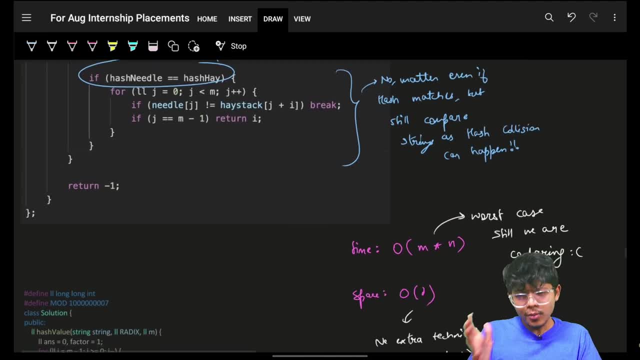 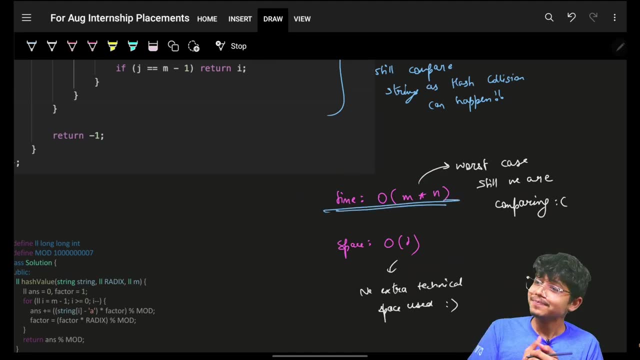 But still there's a high chance. it can be there No matter what, But still, our time complexity will still be same, which is O of M into N. That's a pain, right? Yeah, I know, Uh, but 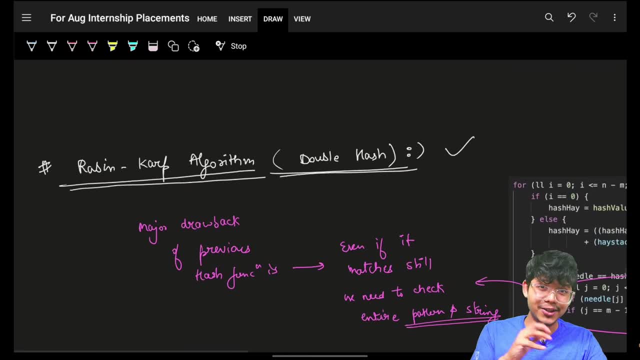 Can we do something? Yeah, we can. So what we can do- I mean, people will not teach this, but the just small thing that you can do is do a double hashing- Exact the same hash function which you use just to do a double hashing. 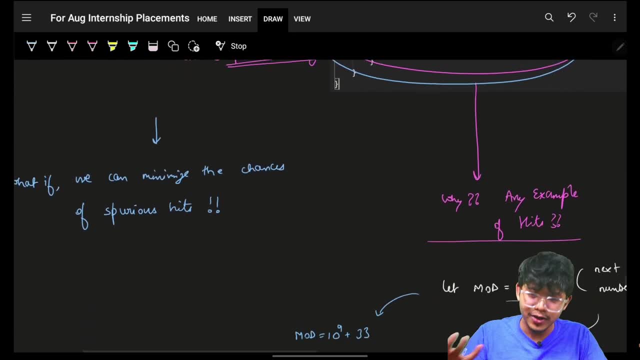 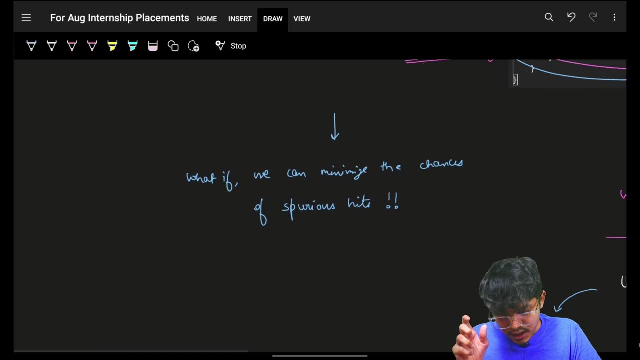 because you know that you will do comparisons that will take again O of M? N time, O of M time again. so that simple thing which you want to want. So do one thing: You have to minimize the chance of spurious hits. You know, you know, you know that you have made this hash function. 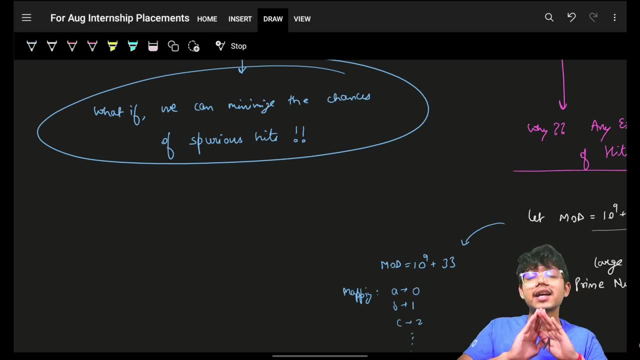 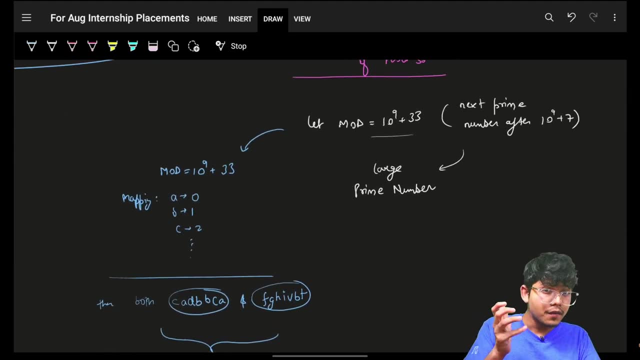 which actually is minimizing the chances of spurious hits, But still there are a lot of chances of your spurious hits being there. So now you will do one thing: What if? what if I told you that there are chances of spurious hits by the above hash function? 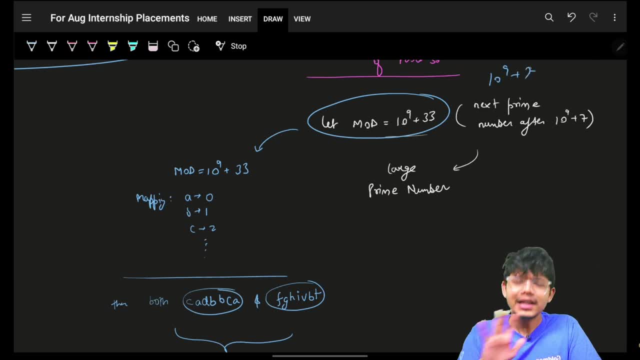 For example, earlier we took the mod as 1 in 97, right, For example, for sake we can take again: that's a prime number, which is a big prime number. I took it as 1 in 97.. 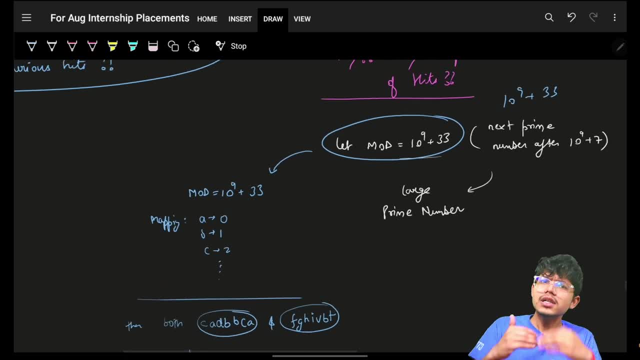 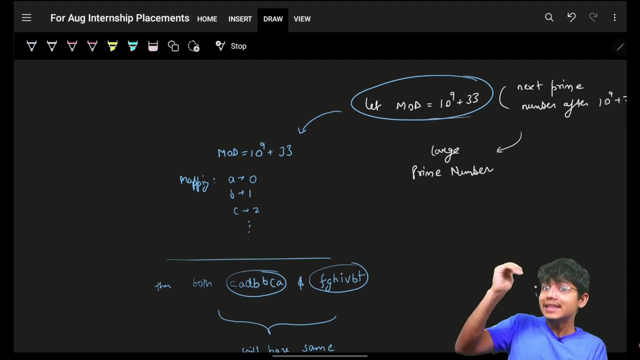 I can still take 1 in 33.. That's also a big prime number, Just after 1 in 97, I can still take that. OK, so let's say again- I'm just showing you an example- with the single hash still you can have a hash collision. 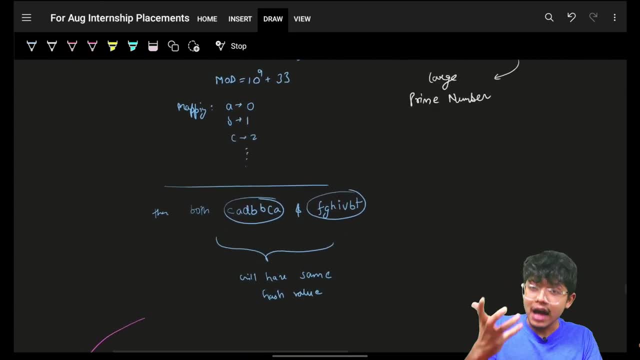 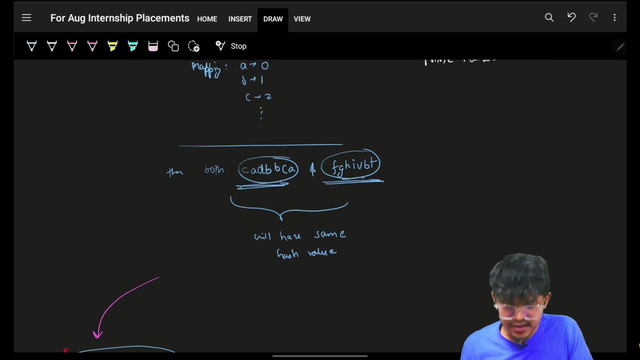 And that's a spurious, spurious hits. So what would have happened is if you had used the mod function like this, then if you had made the hash function of these two strings just correct us their hash function by using this mod operation. 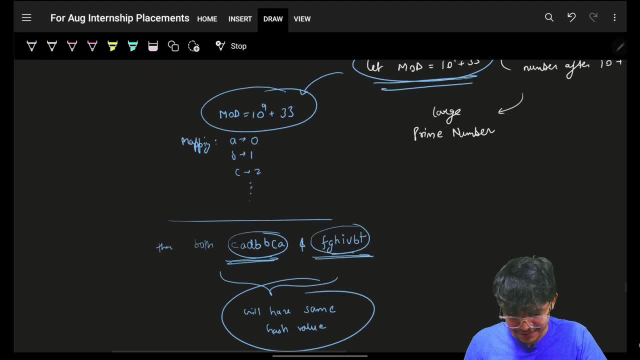 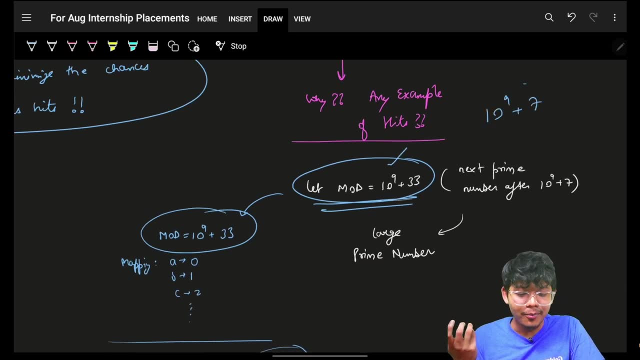 Would have been, would have been seen And you can easily see visibly. they're not at all equal strings. But, Aryan, you use a mod function like this, But you remember we used a mod function of 1 in 97.. 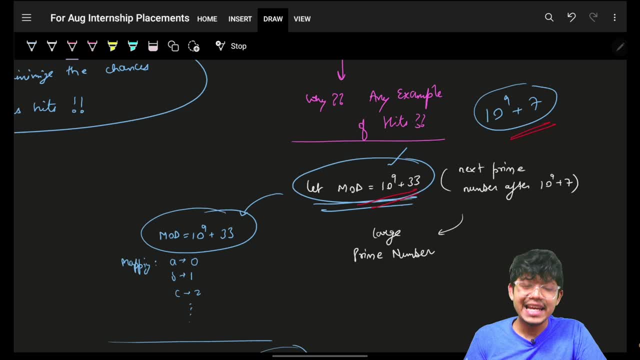 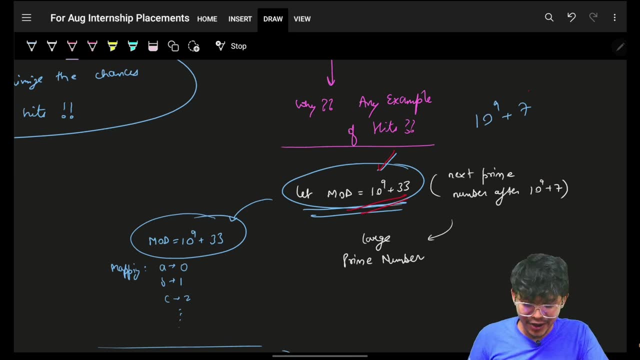 I'll say, bro, both the mod functions have the same identity. How, If I can show you? I can show you an example of this. Why do you think it's not possible to get an example of this also? I can simply write a simple for loop. 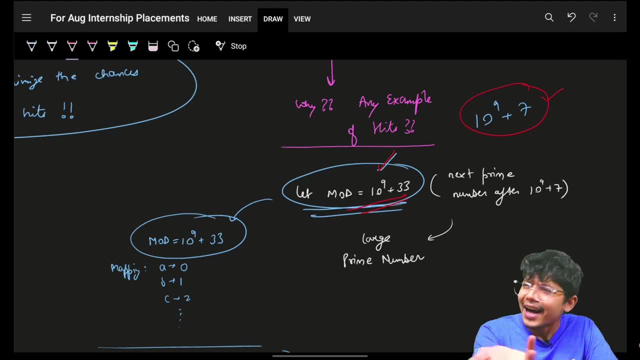 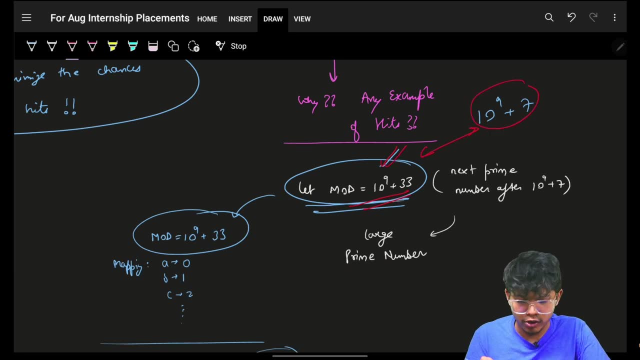 It takes multiple permutations And then can give you an answer. I thought it's a waste of time. So, even if both have the same identity, if this can collide, just this, this can also collide. So this example was for hash, for a mod of 1 in 9 plus 33.. 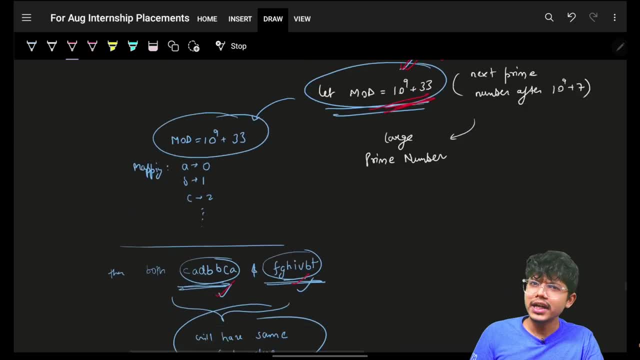 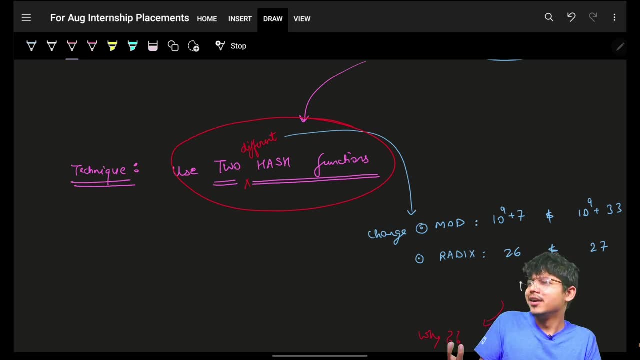 But still with a mod of 1 in 9 plus 7. also it can collide. What's the solution of this Solution is use two different hash function, But Aryan, what's the possibility? Like what's the? what's the thing? 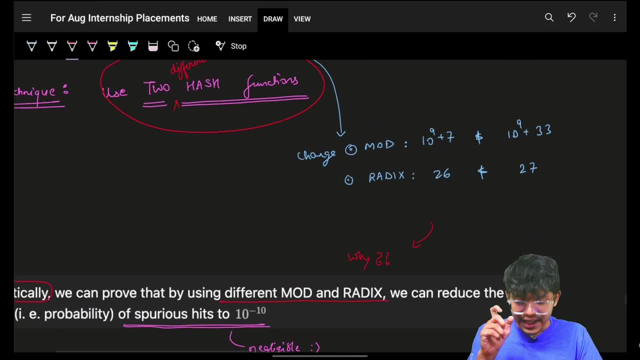 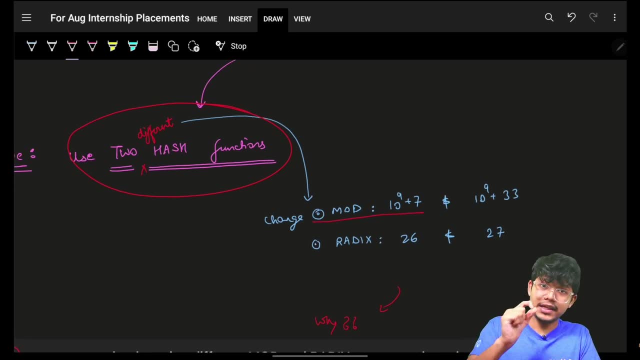 Like why I use it. No, bro, If you will use again. firstly, what it means by using two hash functions. If you remember, we used a mod value of 1 in 9 plus 7 and the and and the value we used of 26,. you remember that part. 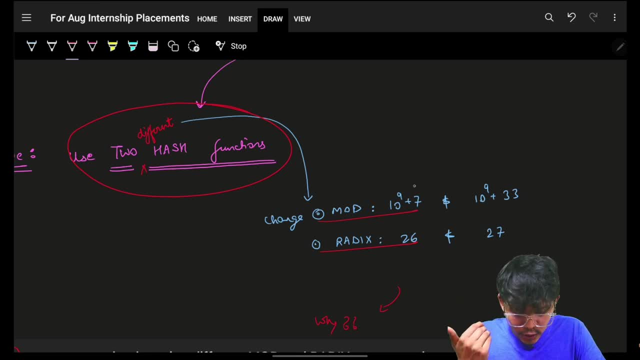 Now I'm saying you should use two hash functions So you can change the mod value to again 1 in 9 plus 33 and then a new Radix value. Again, I told you Radix value can be anything more than 25, which 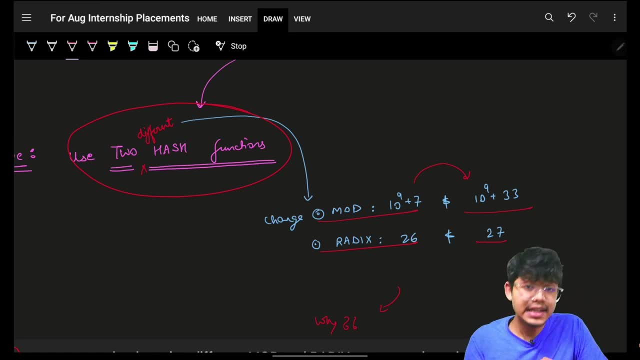 is 26,, 27 and so on and so forth, And we proved that also. So I can take any Radix value. for simplicity, for having a smaller value, We took as 28.. Again, we can take any value bigger value. 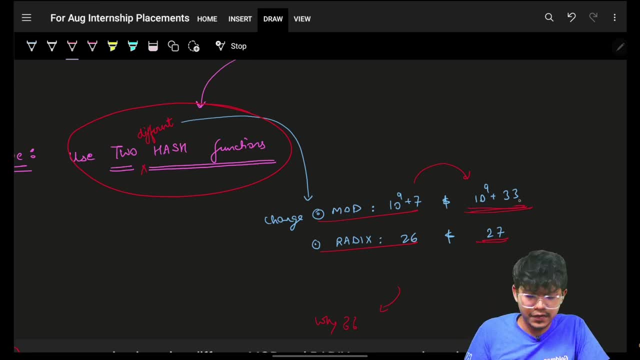 And again we have to take a next, larger prime number, which we take as 29 plus 33.. So now I'm saying I'll compute a hash function by using this, I'll compute a hash function by using this, And now my hash function of needle and haystack should match both with this also. 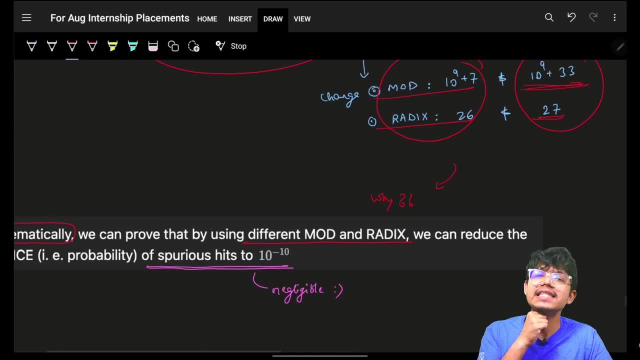 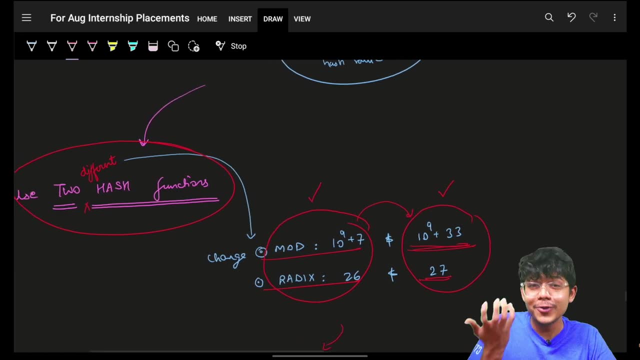 and this also, And then only I can easily say that my hash functions are basically now, then my strings are matching, But, Aryan, still you can have spurious hits. How can you prove that it will not have, bro, Mathematically again, I'm not going to prove also, but mathematically it can be. 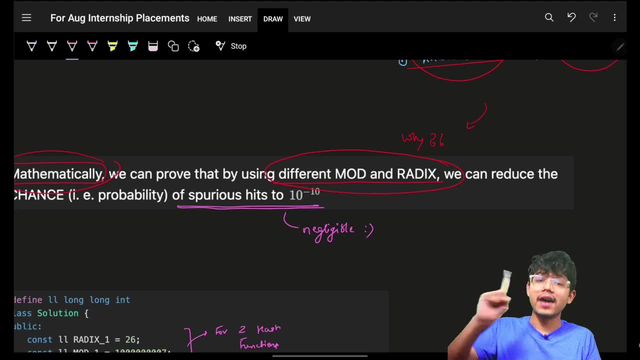 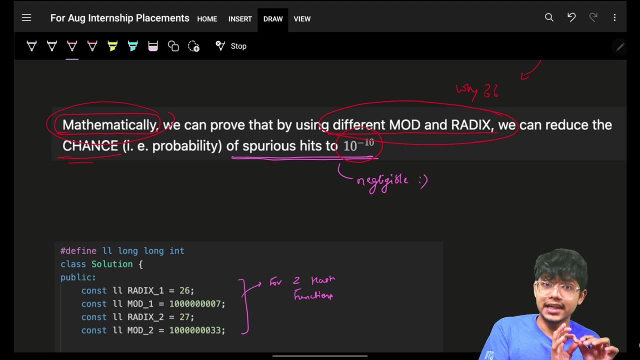 proven that if you use different mod and Radix values, then we can reduce the chance, which is the probability of spurious hits, by 10 nishpa minus a 10. That's a very, very, very, very, very low probability which. 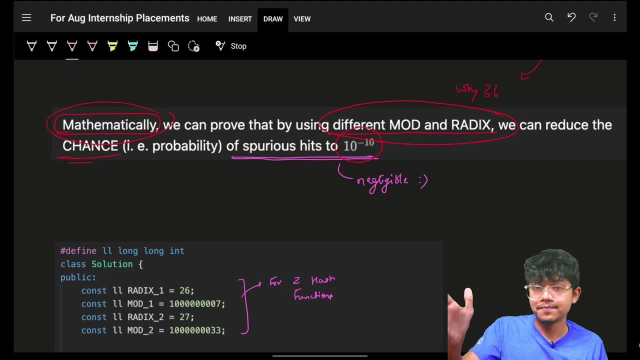 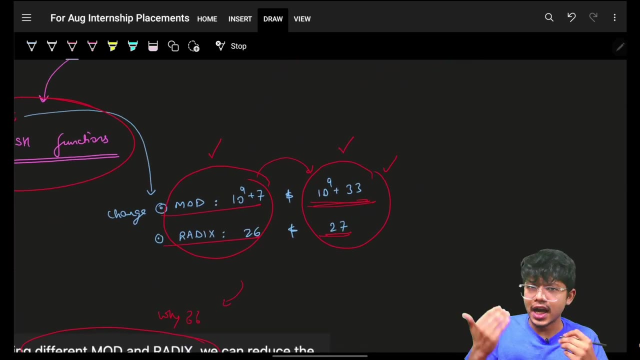 means in the number of test cases the person will write. He has to write So many test cases just to, for just for the probability of that spurious, spurious hit Again. you can, just again, let's say: let's, let's, let's imagine that if, even if you. 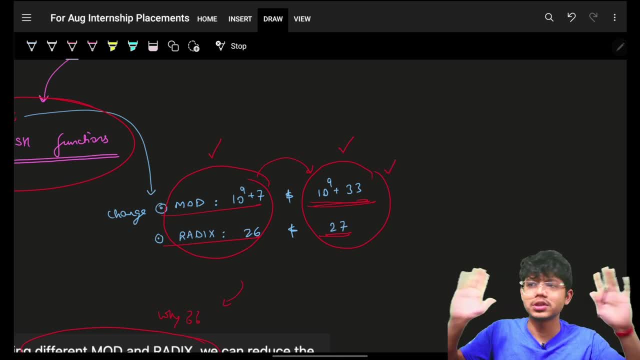 used this hash function again and you know, was possibility, was possibility, but it will, it will. it will never happen, but was possibility. if you use this as this hash function, Right, If you use both of the hash functions and then you're comparing both of them. 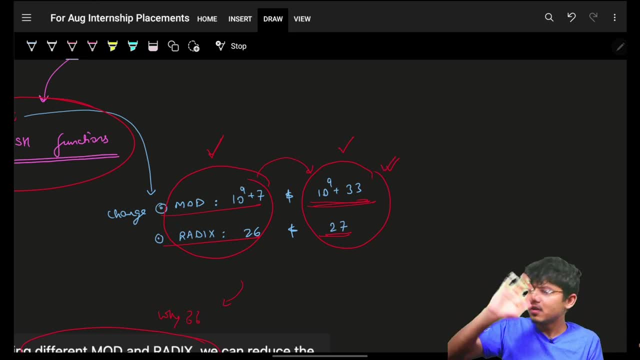 as I'll show you later on. still, if you saw, maybe in future itself it's very highly unlikely, but still very, very, very highly unlikely, But still, let's imagine if you still saw it, just do one thing. 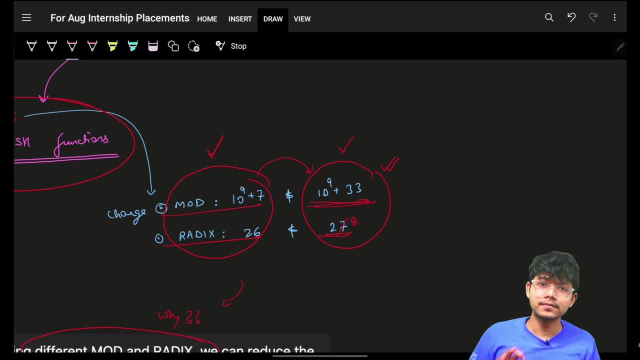 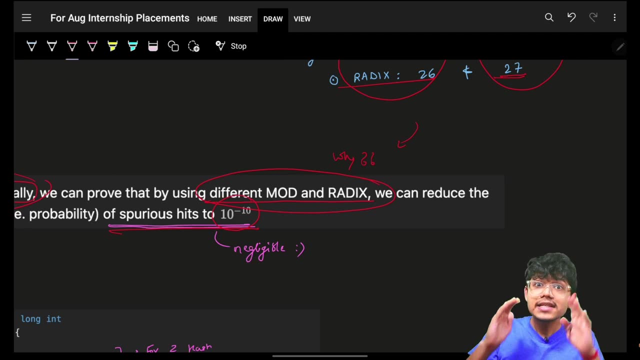 Do just simple one thing: Change this 28.. It will pass, although again I'm saying, it's a very low probability that it will even fail. 10 nishpa minus 10.. Can you just imagine that part? It's a very less probability. 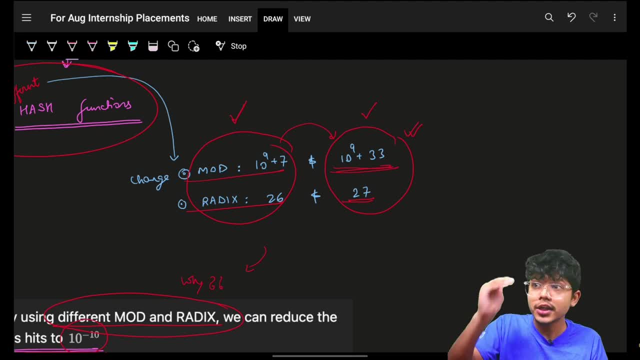 It will fail. Just imagine the person was so into it that he had to make some example that it will fail. Then, bro, do simple one thing. Do it at 28.. Or what if it still fails? Bro, do one thing. 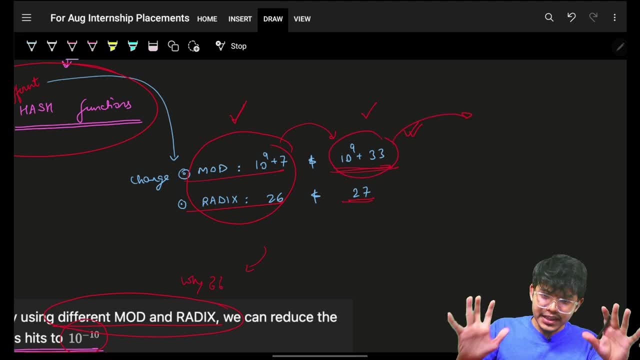 Take the next prime number. Person can never build all the test cases which can actually satisfy this Bro. it will again. Or what if it still fails? bro, Do one thing: Take a next prime number and make another hash, Another, next higher prime number. 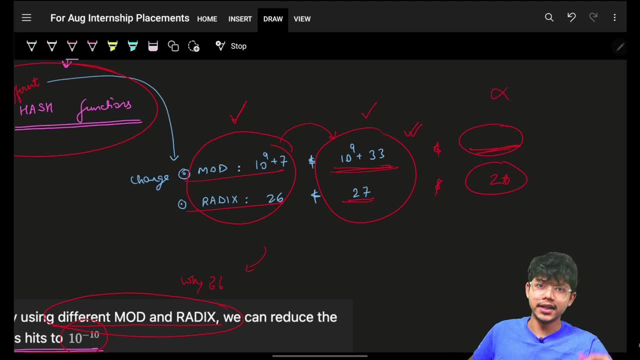 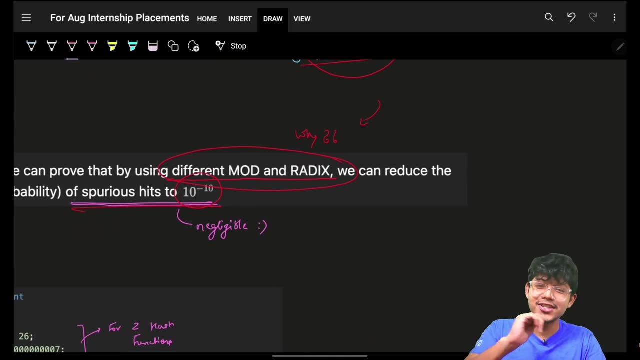 No matter, his even grandfather can not build something like that. So, but yeah, that's a way to extreme for the folks who are actually about to fight me. So for them only, I just told you a solution, But still, no matter what, you can never reach to this superior set. 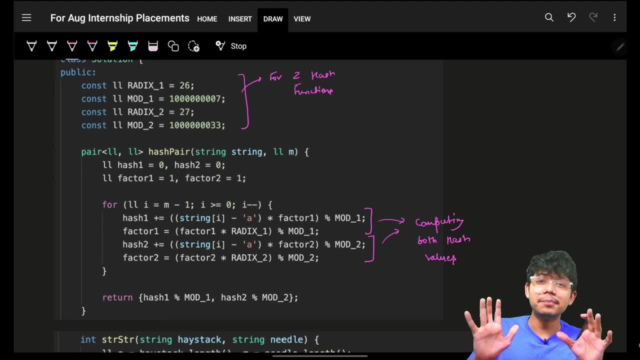 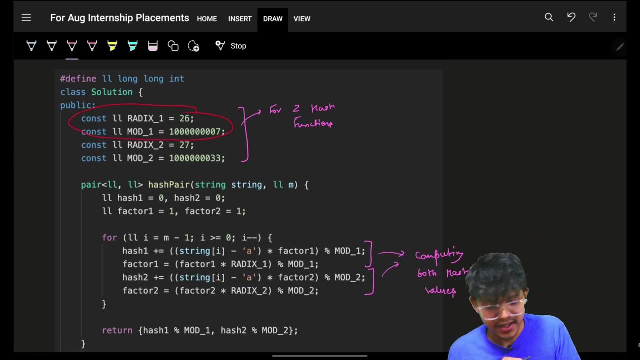 It is very, very negligible. So what's the change in this Simple Two red X value, two mod values. So I will have a red X value one as 26,, mod value as 19 plus 7.. Red X value two as 27 and mod value as 19 plus 33.. 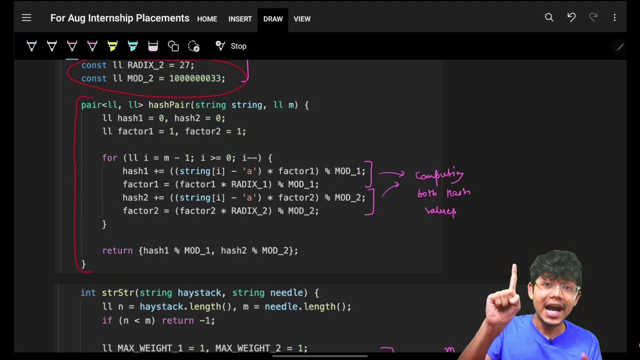 Now hash function. Now, instead of returning one hash, I will return two hashes. Exact same thing will go on, Just both of them. I will be computing now. So again you will see factor. I had only earlier factor one. 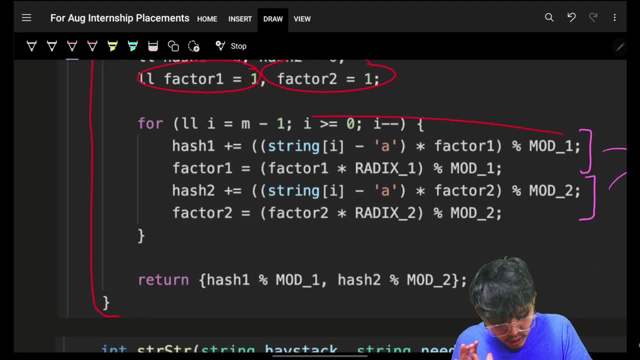 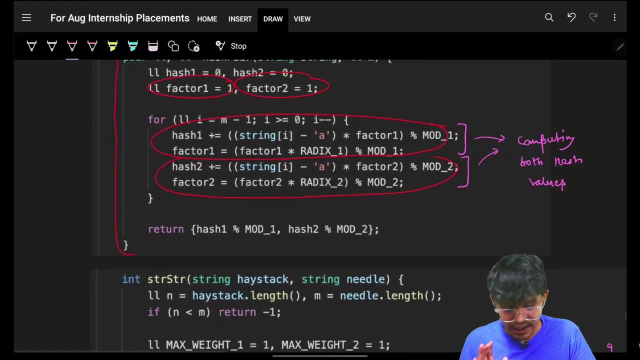 Now just another factor: factor two was also added. So earlier I had only this computation of hash and factor, hash one and factor one. Now I'll also compute hash two and factor two, Only returning hash one. Now I'll return both hash one and hash two. 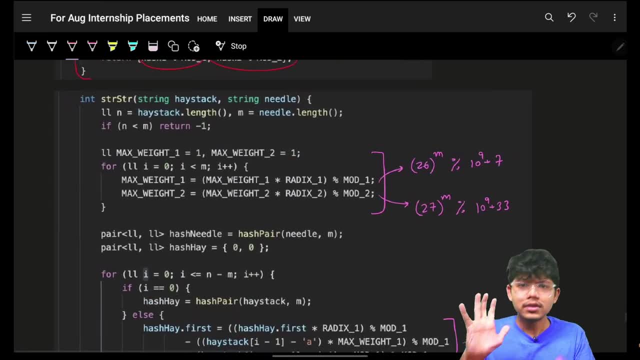 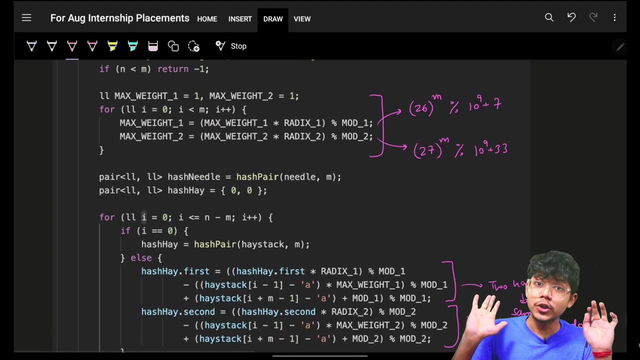 That's how I'll simply keep on going about it. Now, simple, it's the same thing in the code. also, Basic condition: if what if needle size is more? if it is less, then you can go about it. Now you have to compute max weight. 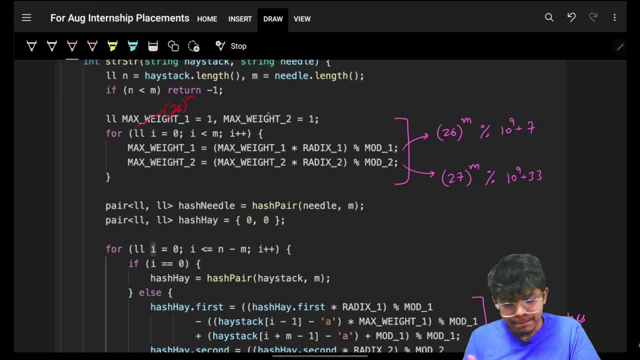 Earlier max weight was 26 ratio power m. Now max weight two will be 27 ratio power m, So I have to compute both of them. So I'll compute both of them, but with their corresponding mod values. Make sure that part. 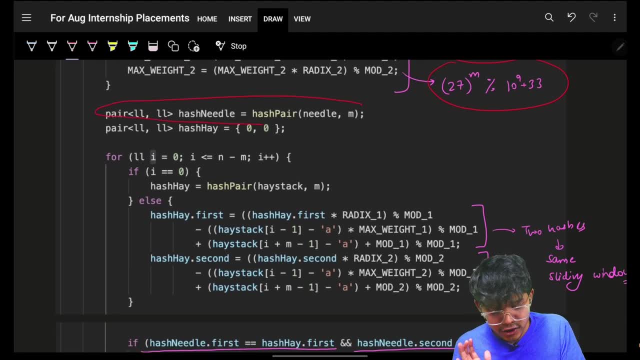 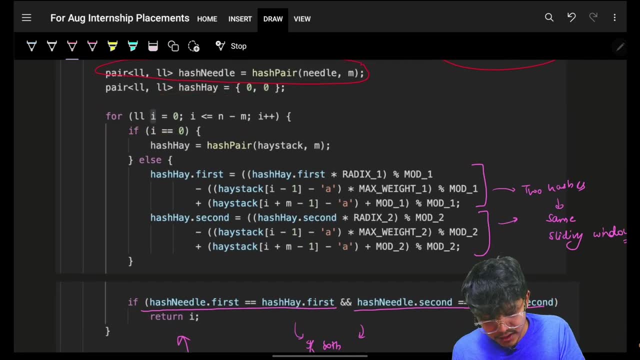 OK, when this is done- now you have got the hash of the needle as a pair, both the hashes you have got- then you will simply keep on going Again. exact same thing. exact same thing. Now you are again, it's just that earlier hash was simply a long long. 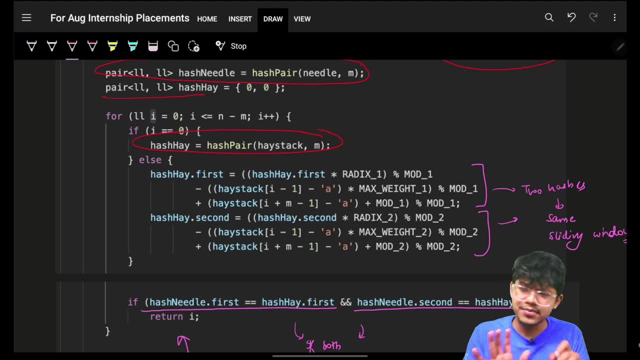 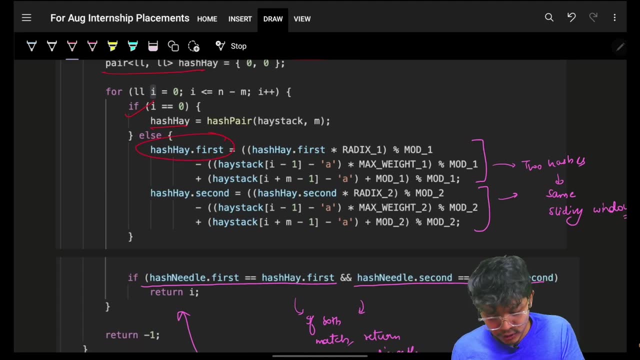 Now it's a pair of long long. So now you just simply again exact same stuff. Get the hash here for the i equal to zero. For the other hashes you just use the sliding window. For the sliding window I'll compute the hash first, the hash second. 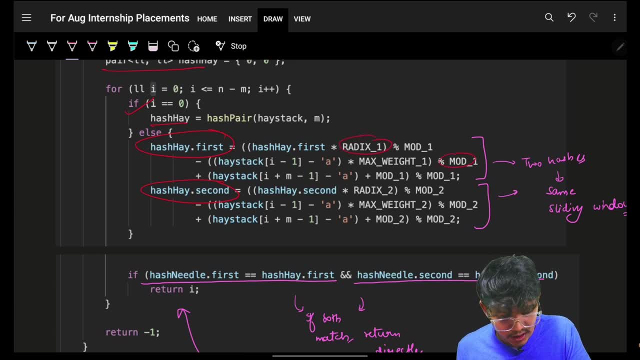 Again exact same stuff, Just using the radix one mod one, radix two and the max weight two and stuff For the hash two. use radix two, max weight two, mod two and so on and so forth, When you have got hash one and like hash first and hash second. 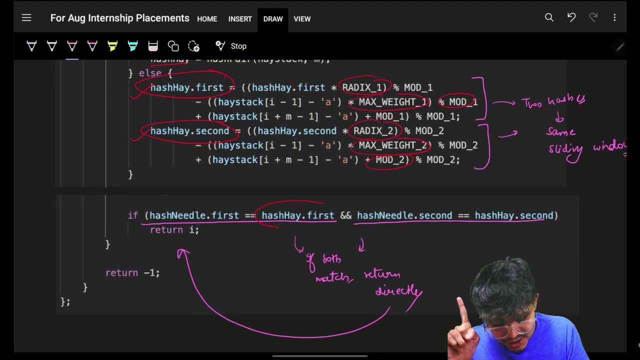 compare both of them and both of them should be equal. So hash here first, which means hash of haystack first, which means the first hash and the first hash of needle should be same. The second hash of needle and the second hash of haystack should be same. 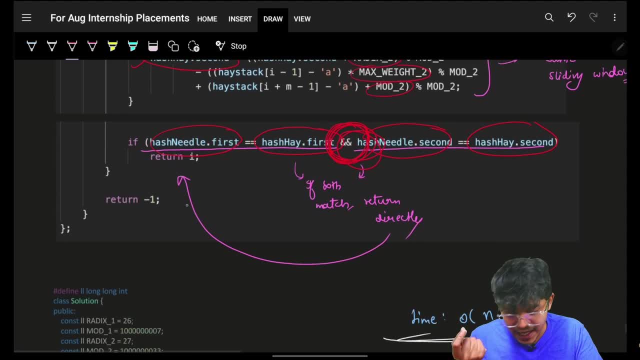 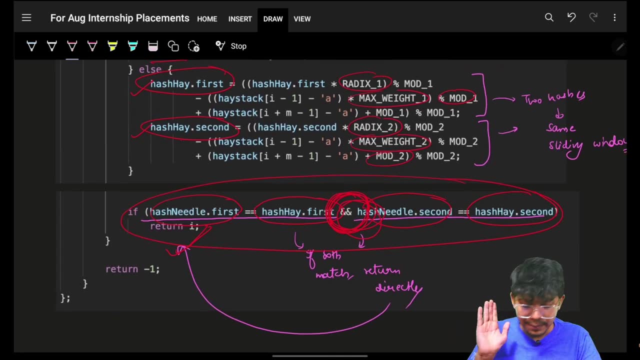 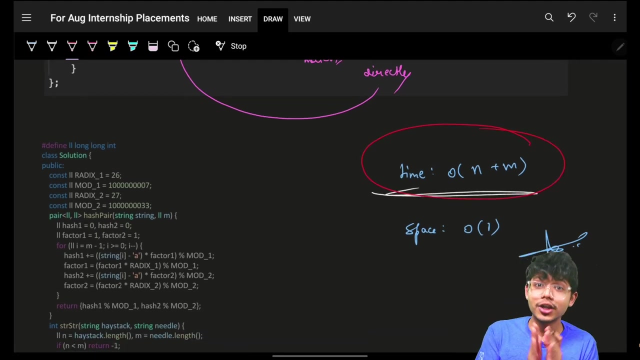 Both of them should be same. only then I'll say that it is the matching one, If it is not simply return. So you saw the extra thing which I was comparing here. It is gone by simply computing a second hash function, And that's how my time complexity is now O of n plus m and not O of n into m. 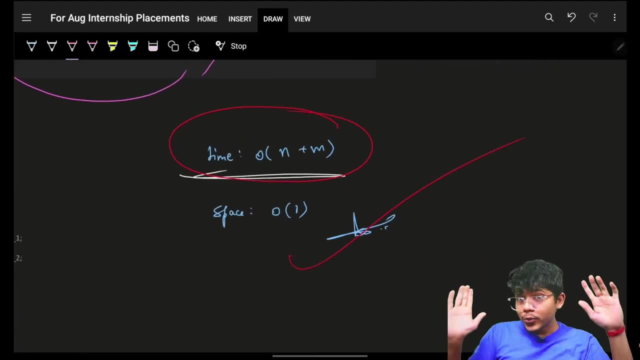 And that's how you can simply solve it. Again, you will never get spurious hits if, even if you get it, please simply update the radix value to 28.. It will solve it Still. you get it. Firstly, you will never get it. 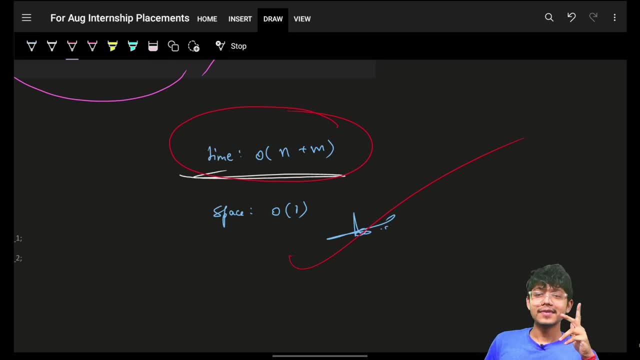 But still if you move it to 29.. If you are thinking, oh, I always ICPC, World Finals, bro, do one thing, make another hash function and then compare all three hashes. That's it Cool. I hope that you guys got the entire Rabin Cup. 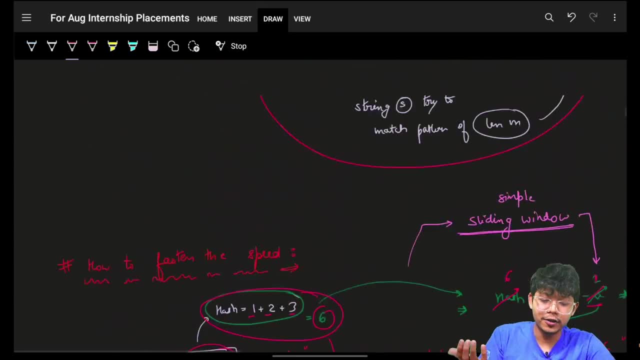 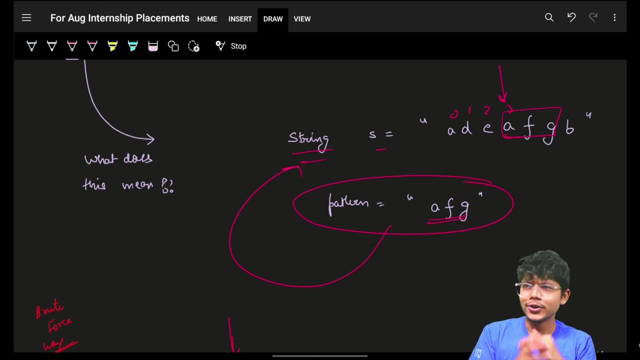 People were actually going mad about. I had to bring it as a part of 100 days- 100 days challenge, but it was way too much hectic for me So I had to bring it this video first. I'll keep bringing in the 100 days- 100k later on Cool. Bye, bye, Thank you so much. Goodbye, Take care And thank you for watching.